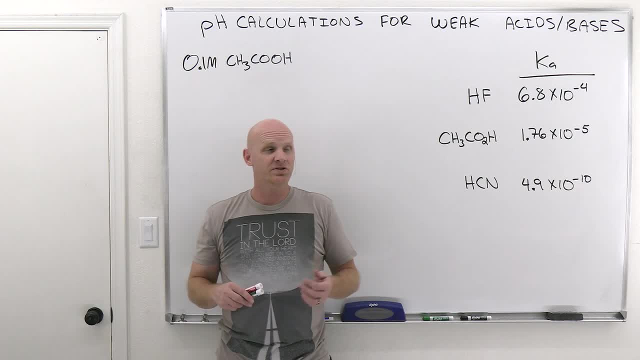 subscribe to the channel. click the bell notification. All right, so we're going to start off with weak acids, We'll move on to weak bases and you'll find that this really quickly. this is a much bigger pain in the butt than what we dealt with with strong acids. So really quickly. 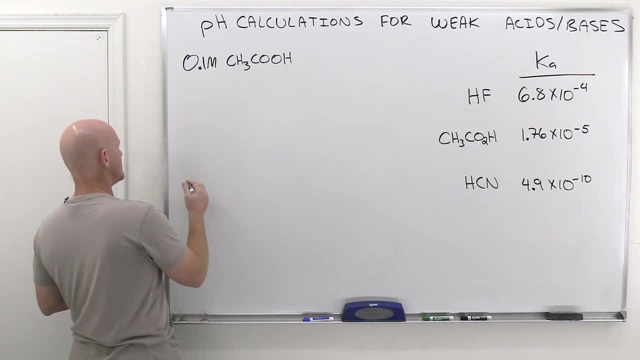 I want to review strong acids for just a second. So we looked at, say, you know, 0.1 molar HCl in the last lesson and it dissociated 100% into H plus and Cl minus. And because it dissociated 100% we could very quickly and very easily rationalize that the H plus 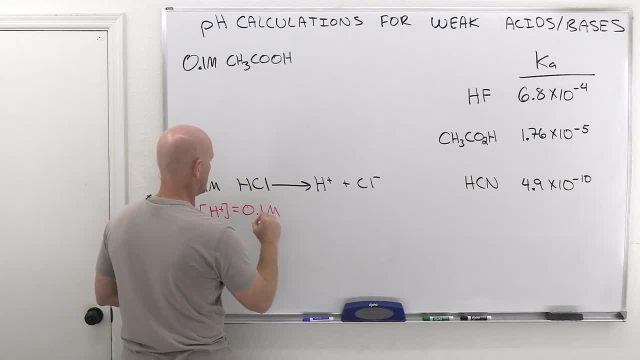 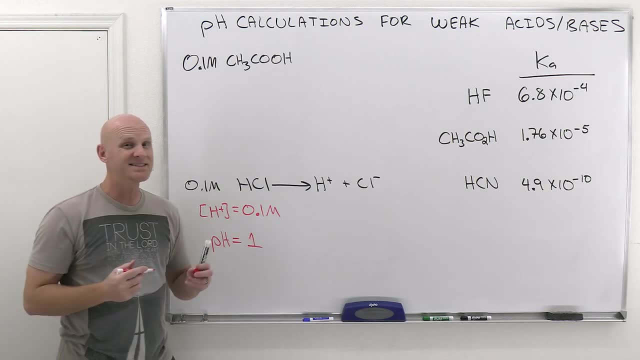 concentration 1 to 1 ratio was just going to equal 0.1 molar, And then the pH, which is simply the negative log of that, was equal to 1. And we can come out with a pH in like 10 seconds. 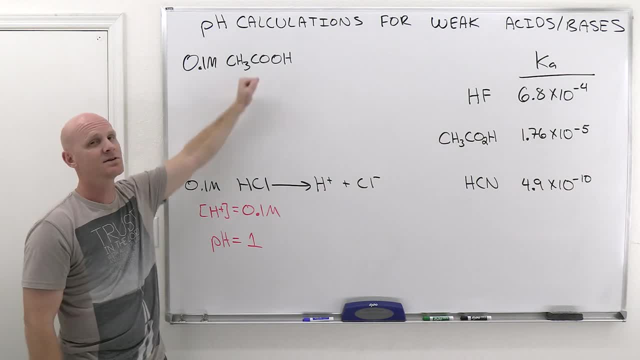 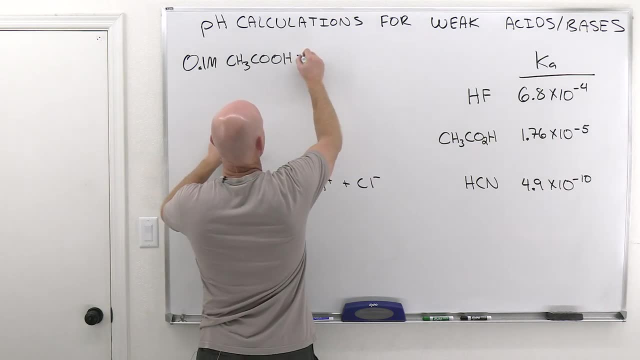 15 seconds. It is not going to be the case initially, for weak acids in this case. So here I've got 0.1 molar acetic acid. So an acetic acid unfortunately does not dissociate completely, It only dissociates partially. 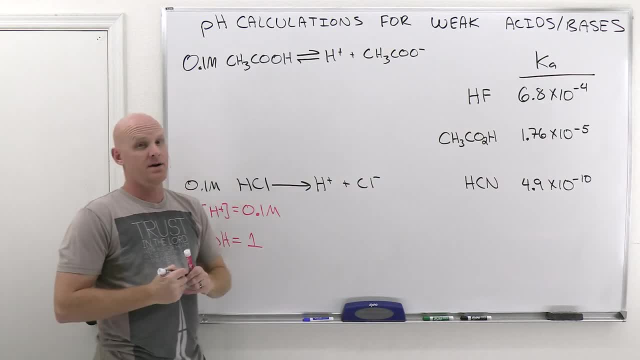 And so the question is: how much H plus do you get? Well, I don't know off the top of my head, But what I can tell you is this: The H plus concentration does not equal 0.1 molar because it does not dissociate. 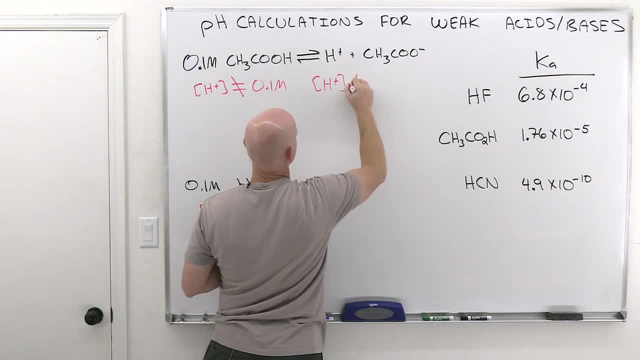 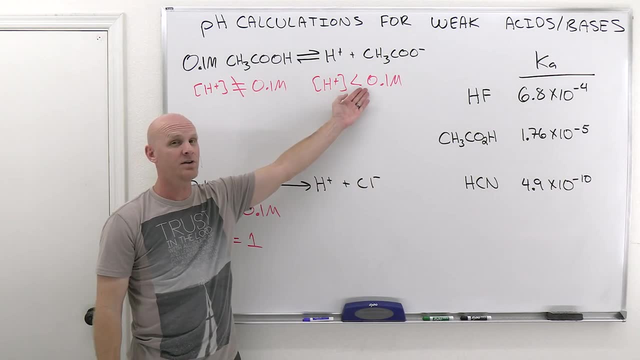 completely. In fact, we could take that a step further and say that the H plus concentration is going to be less than 0.1 molar, And in fact we could take that even a step further and say that it's probably going to be considerably less than 0.1 molar, since a typical weak acid is going. 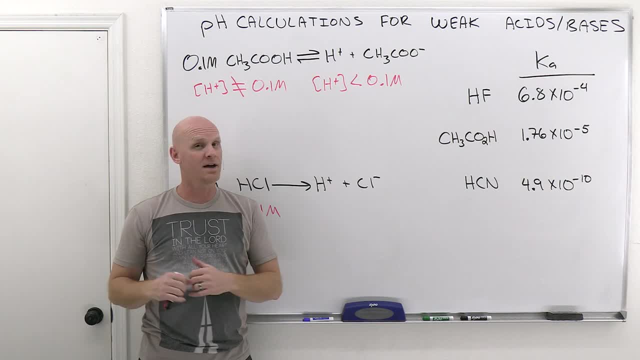 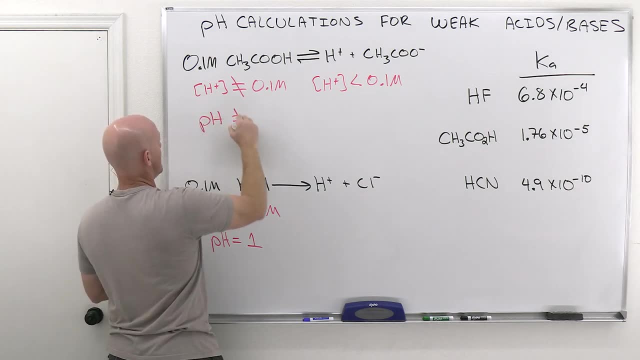 to dissociate less than 5% and, on the other hand, it's going to be less than 0.1 molar, Alright, so what does that also mean in terms of pH? What DOES that also mean is that your pH does not equal 1.. 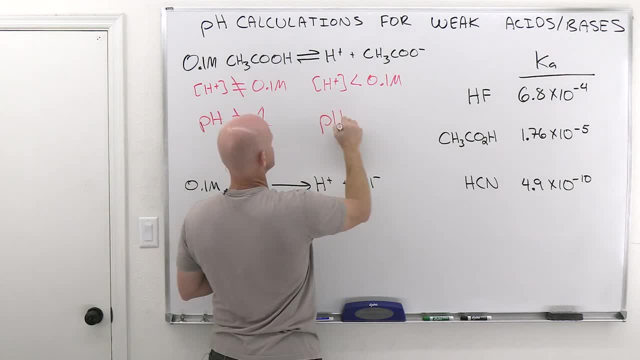 It's going to be nowhere near as acidic as 1.. So your pH in this case is going to be greater than 1.. Just keep in mind this inverse relationship: As your H plus concentration goes down, your pH is going to go up, Since we knew the H plus is less than 0.1,. 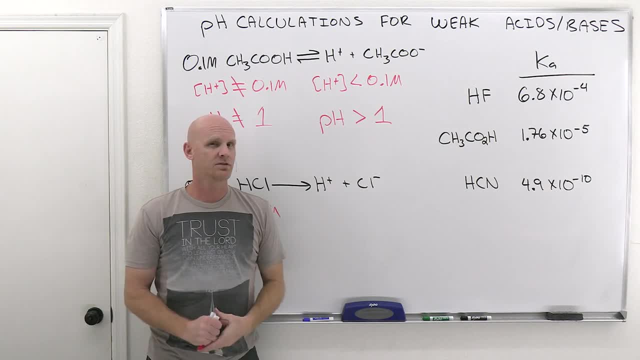 that means the pH is going to be greater than 1.. So, anyway, not too happy with that idea. Now, remember, we've only said said what it's not equal to, but we haven't actually, like come out with a plan to figure. 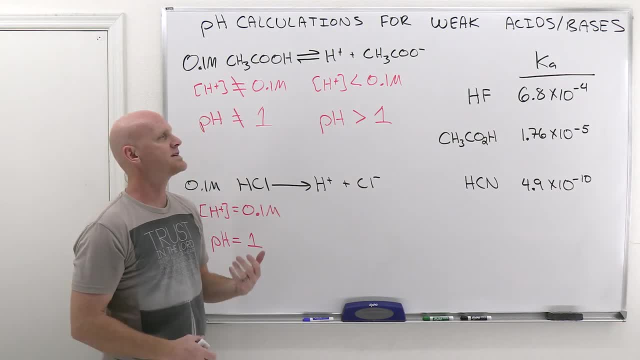 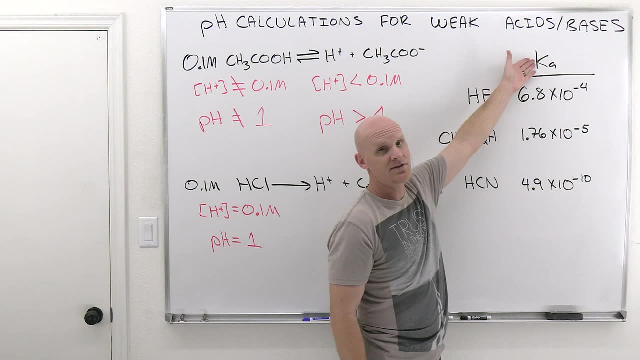 out. what is the pH exactly going to be equal to? Well, it turns out we need a little more info, And that info is going to be what we call a Ka expression and a Ka value in this case, And Ka is just an equilibrium constant, And it is an equilibrium constant specifically for when a 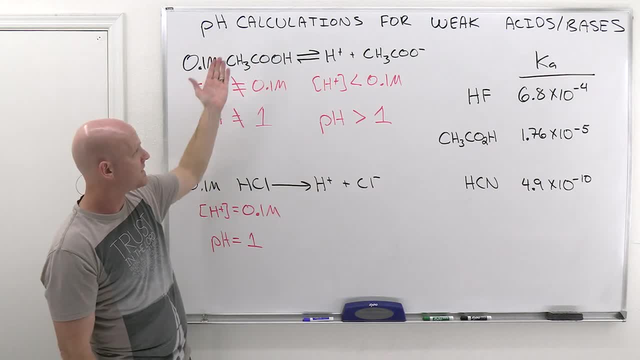 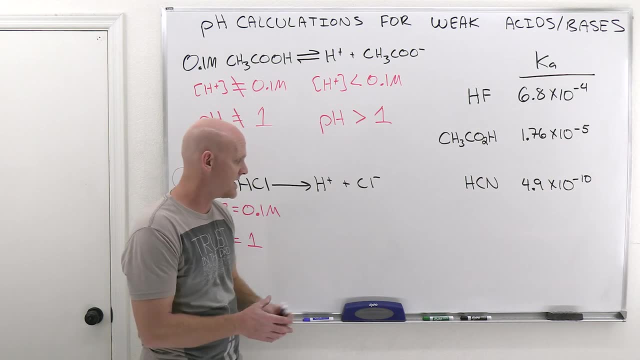 weak acid dissociates, And so in the case of acetic acid, we can see here this is another way of writing acetic acid. The Ka value is 1.76 times 10 to the negative five. So and we're going. 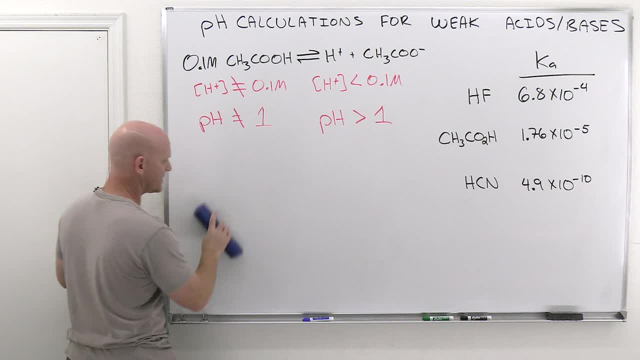 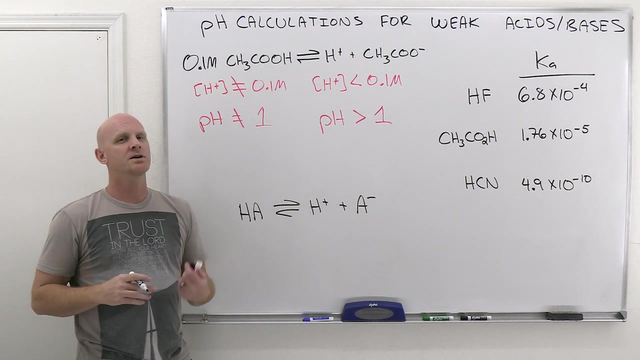 to write this generically for any you know kind of standard weak acid here. So in this case, instead of writing acetic acid, I'm just going to write this generically for Ha, dissociating to give H plus and A minus, And some people prefer to show the water. We talked in a couple of lessons. 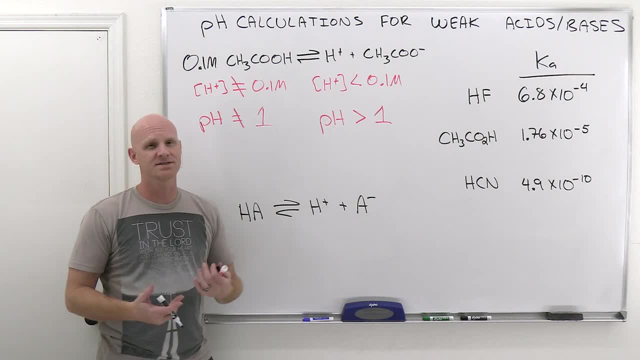 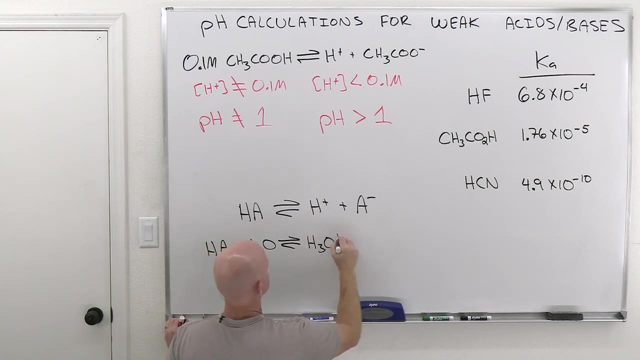 ago that H plus indicates what we call naked protons, And it's so reactive that it probably doesn't exist in water. It probably actually exists as some form of H3O plus instead, And so you could also write this reaction as Ha plus water giving H3O plus. 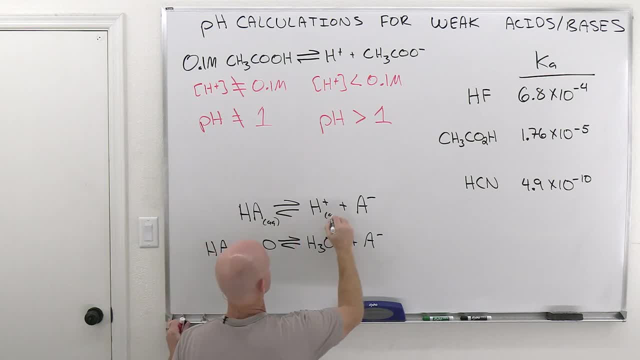 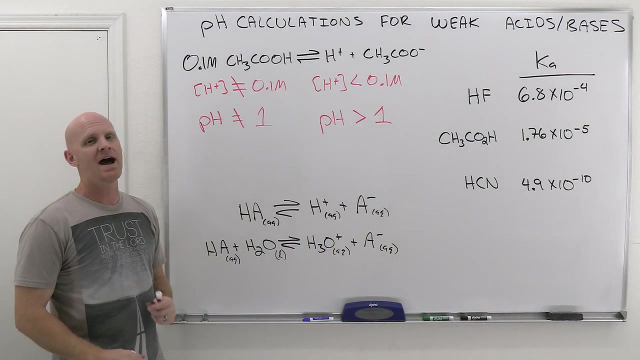 plus A, minus the conjugate base. If we label our phases got water as the only liquid, everything else is aqueous, And so the equilibrium constant for this generic reaction of a weak acid dissociating, that's what we refer to as Ka. 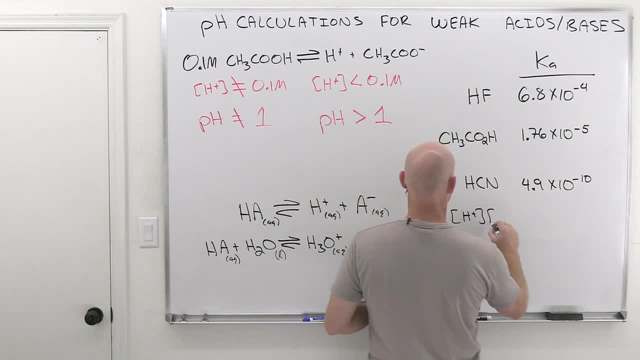 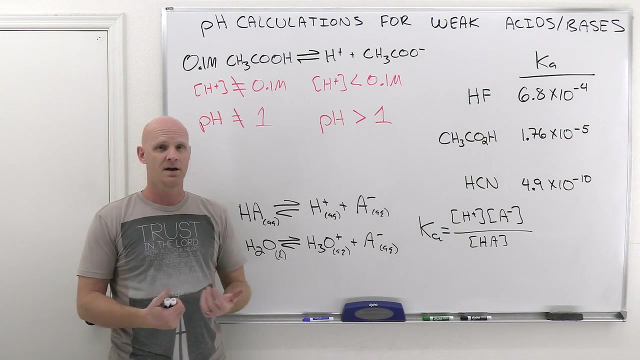 And so for the top one here we'd write H plus times A minus all over Ha. If you did it for the bottom one, notice instead of H plus on top you'd write H3O plus. We treat those as synonymous H plus hydronion concentration or H3O plus hydronium. 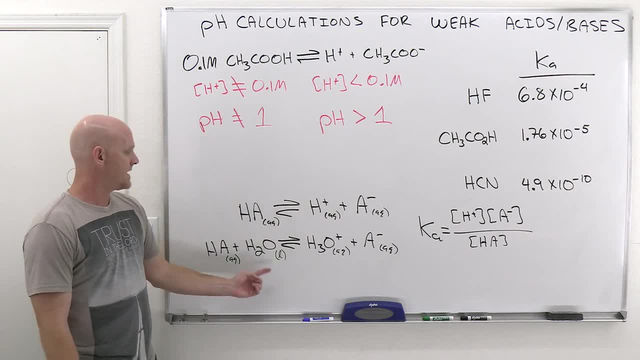 concentration, Totally analogous. So we're going to write H plus times A, minus all over Ha, Totally equivalent. And in this case we'd leave the water out anyways, because it's a liquid and no solids. no liquids in your equilibrium: constant expression. So just products over reactants. 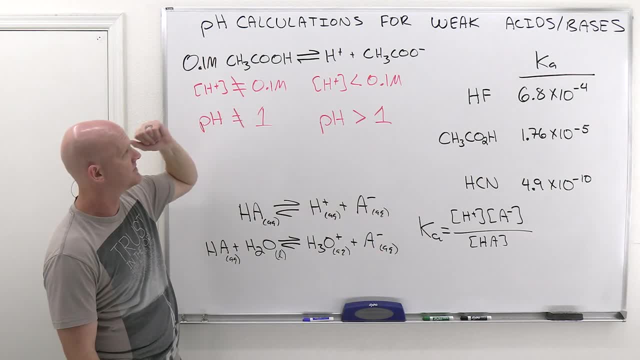 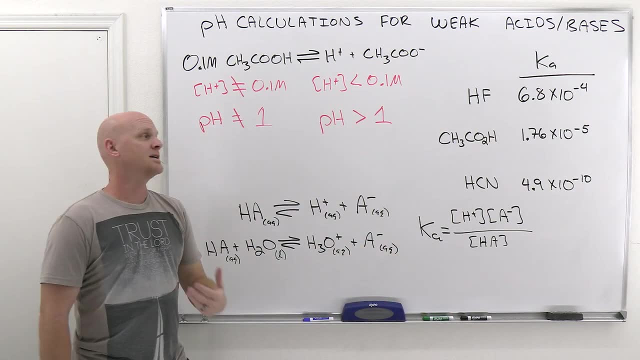 So this is generically a Ka. If you do this for acetic acid, instead of A minus you'd have CH3COO minus, And instead of Ha you'd have CH3COOH. If you did this for, say, HF, then instead of A minus. 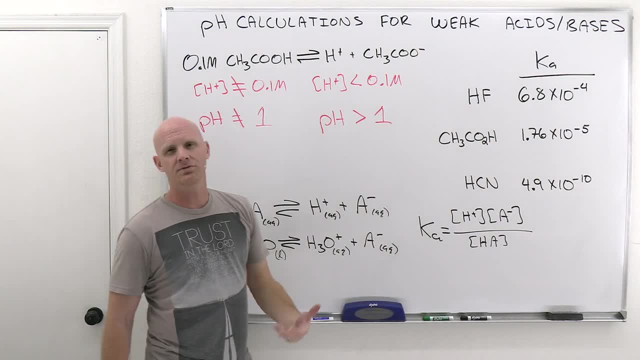 you'd have F minus, And instead of Ha you'd have HF, So on and so forth. You should know how to write this dissociation reaction, with or without H3O plus. And if you did this for H3O plus, you'd. 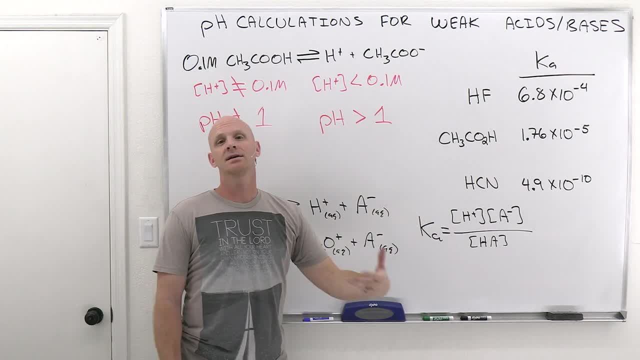 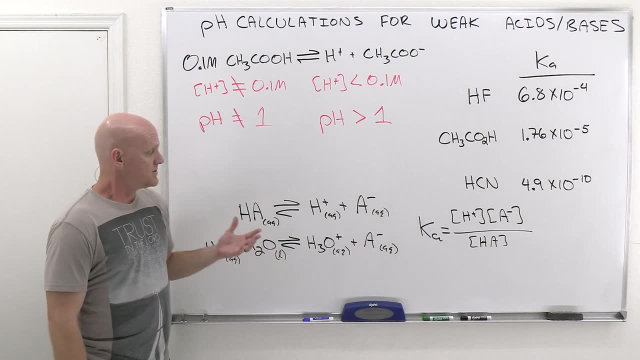 or without water, And you should be able to write the Ka expression for any given weak acid: I provide you or anybody provides you. All right. So if you look at this equilibrium constant, so an acid is measured as its strength based on how much it dissociates. The greater it dissociates, the 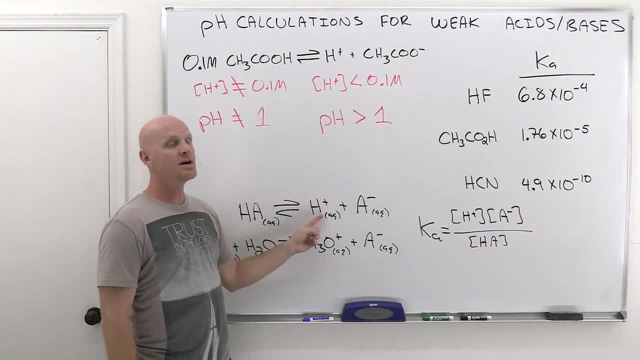 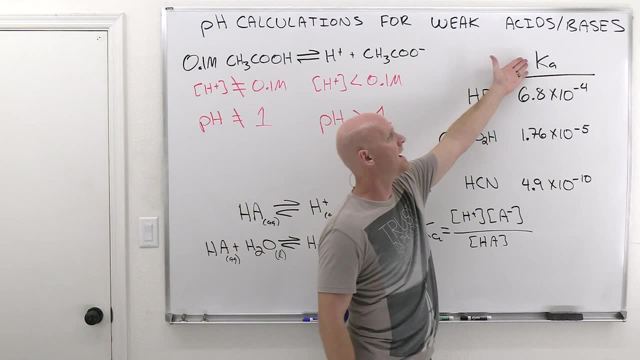 stronger we say that acid is, And if it dissociates more, you're going to get more products. And if you get more products, that means you have a higher equilibrium constant. And so now we have a single value, the Ka value. that'll give us an idea. 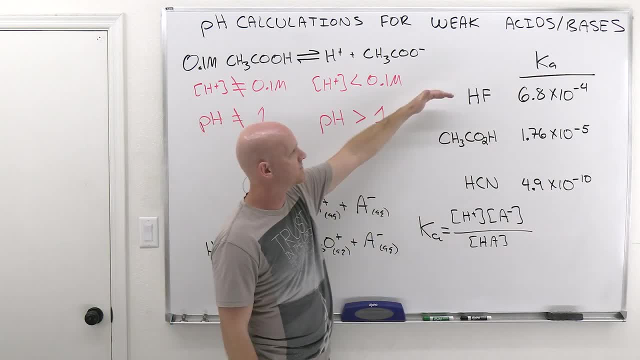 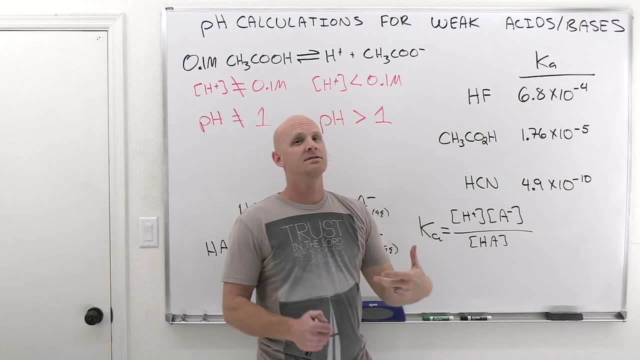 How strong this acid is, at least relatively speaking. And so here I've got three acids. I've got a hydrofluoric acid, acetic acid and hydrocyanic acid, And I've provided you with their Ka values, And from this you could look at this and say, oh, HF is the strongest of these. 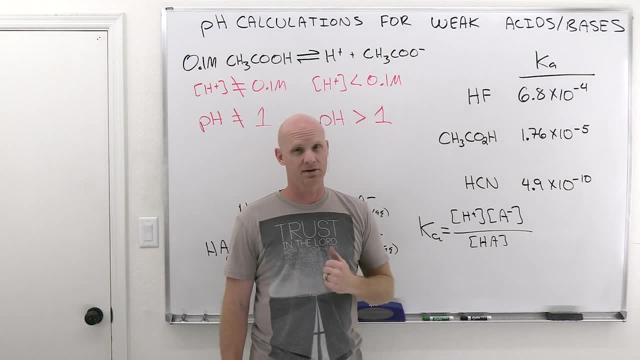 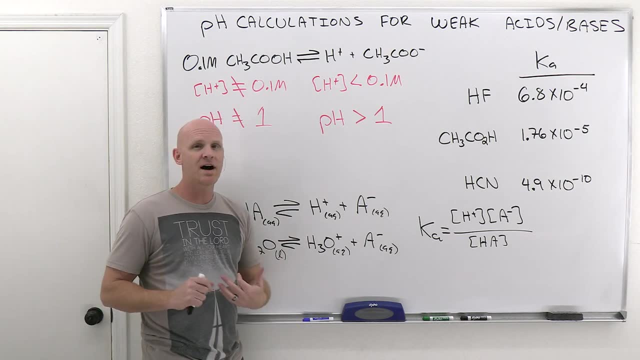 three weak acids, And HCN is the weakest of these three weak acids. So just by comparing their Ka values, we now have a measure, a numerical value that allows us to compare the relative acidities of all these different weak acids. So that's great. 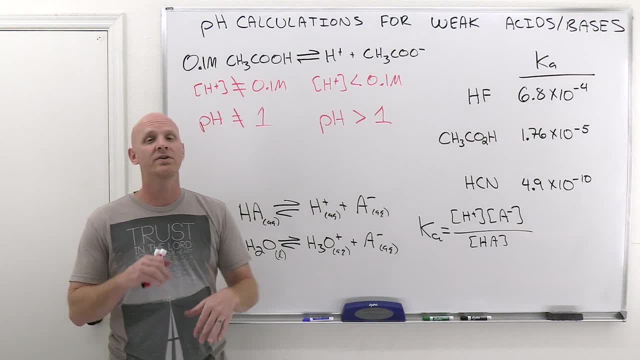 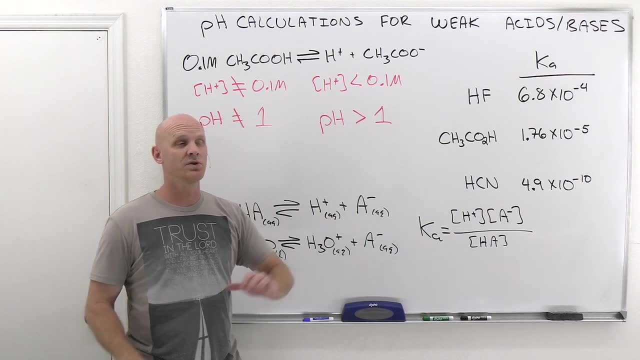 Earlier in the chapter we learned how to compare relative acidities for binary acids and for oxoacids and for the different acids in a polyprotic acid sequence, And that was very conceptual. Now we've got a numerical estimation for comparing any two weak acids, as long as you know their Ka. 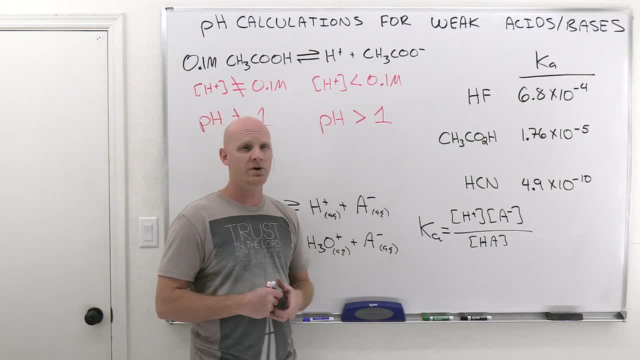 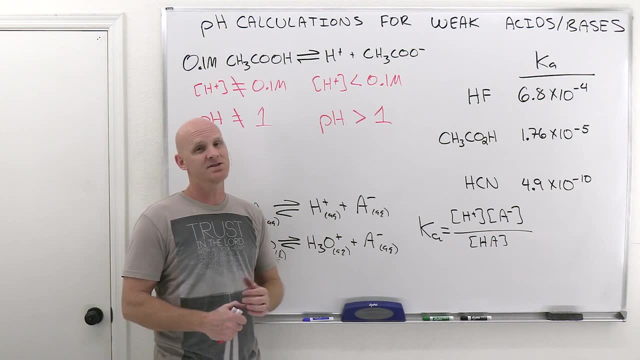 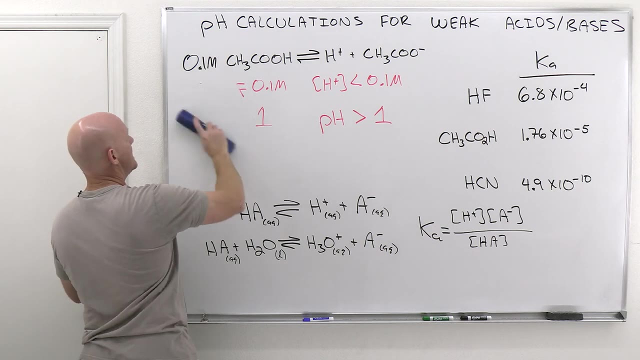 values. Whichever one has, the higher Ka value is the stronger of those two acids. Okay, And it's this Ka value also that's going to allow us to calculate the pH in the end. but it's going to be a much bigger pain in the butt, as we're about to see here. So we're going to go back and do this. 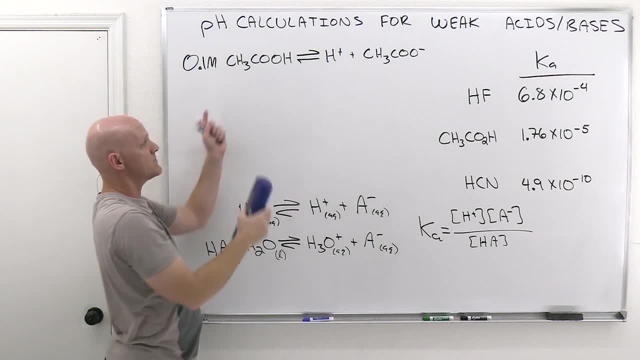 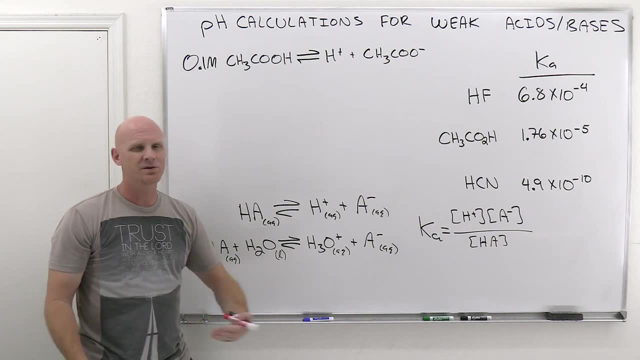 for acetic acid, but I'm going to write this out generically. So instead of doing this specifically, I'm actually going to work it generically. for any weak, we say monoprotic acid with just one H. Well, you're only going to be dealing with one H at a time in any example you see in this course. 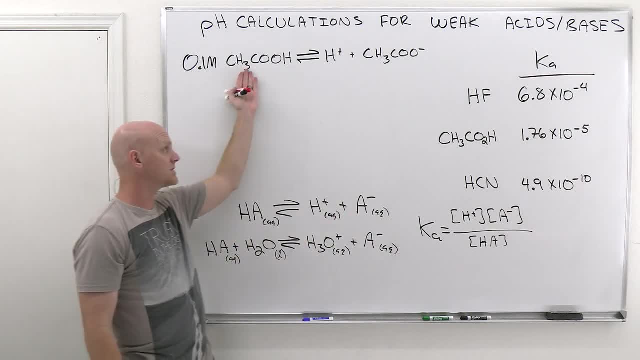 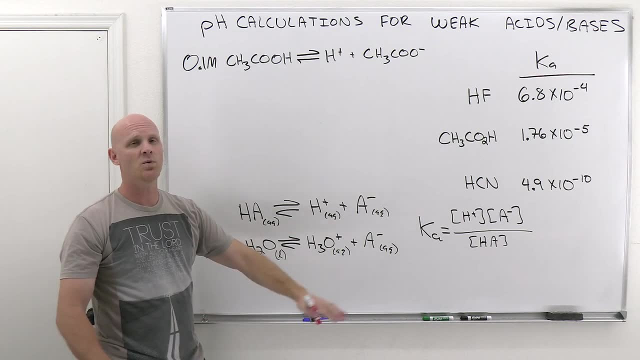 So for any weak acid you can just use this generic expression. You don't actually actually write out your specific acids. dissociation reaction: You can keep it generic And the calculations will work the same way every time. Let's take a look. All right, So the first actual 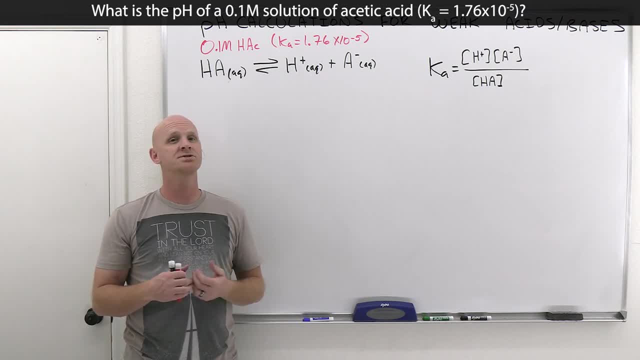 calculation we're going to perform is to find the pH of a 0.1 molar solution of acetic acid, And I'll write acetic acid generically like this. I'll abbreviate it this way: The Ka is given as 1.76. 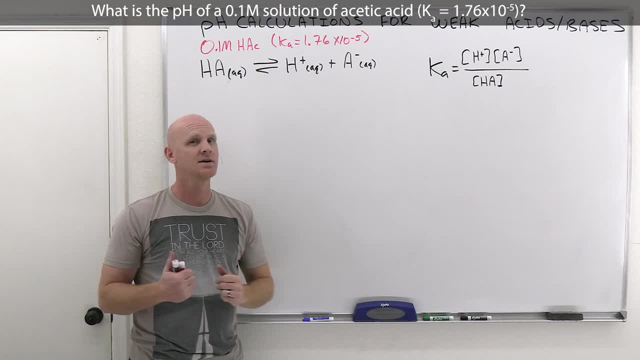 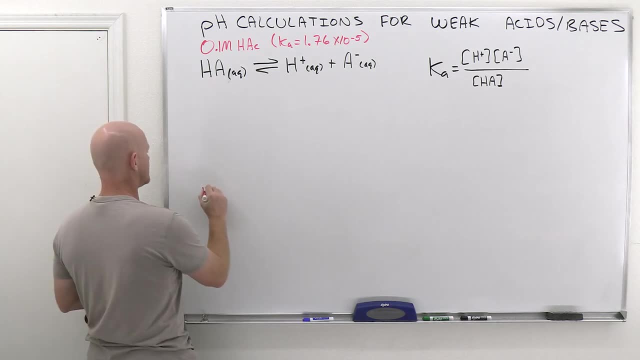 times 10 to the negative five. That's also provided. It had to be provided, as we'll see here, And in this case it can be a little bit pain in the butt. And just again, one more quick reminder Again: if you've got a strong acid, it's going to dissociate 100%. 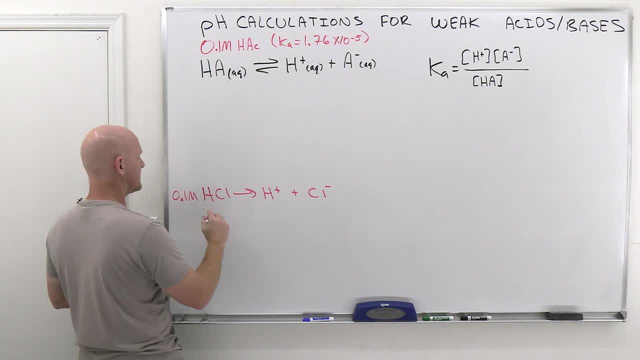 so if we had 0.1 molar HCl, well, that means you're going to end up with an H plus concentration of 0.1 molar, and you'll just simply take the negative log of 0.1 to get the pH. 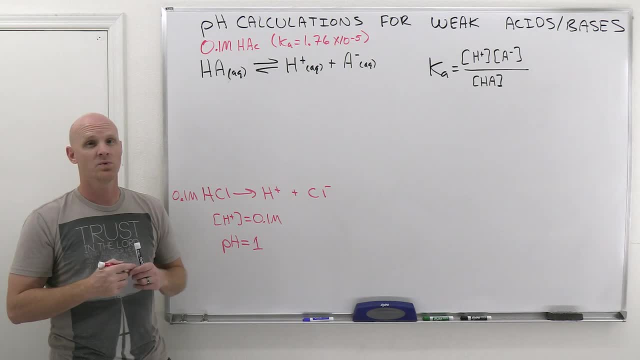 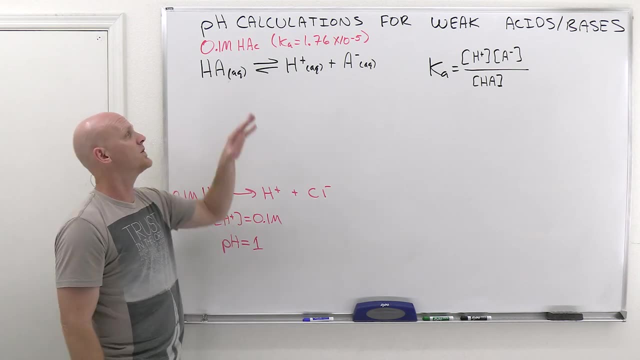 and it's going to simply equal one. So life is good. Strong acid really easy. You know it dissociates completely and that makes figuring out how much H plus you have in your solution really simple, really straightforward. With the weak acid, not so much. It doesn't dissociate completely. 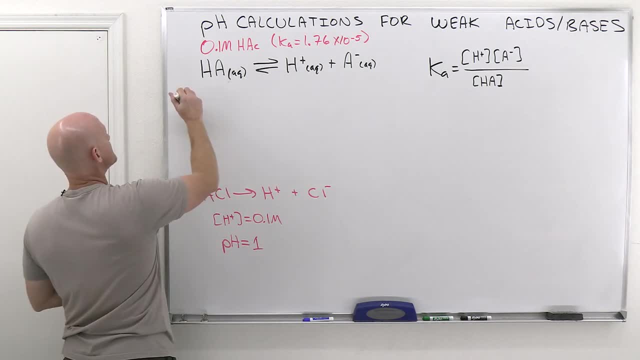 Finding out how much H plus you have. it's going to be a little bit of a process. It's going to reach some sort of H plus. It's going to be a little bit of a process. It's going to reach some sort of. 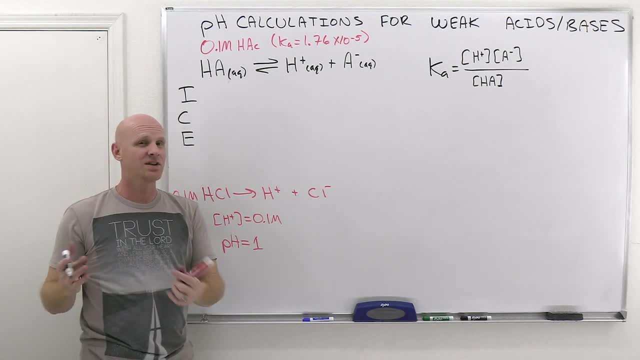 intermediate equilibrium and we're going to use one of those ice tables, one of those ice charts to figure out how much H plus do we have at equilibrium. So the whole goal of setting up the ice table and everything is, if we're doing a pH calculation- is- I don't need to know what. 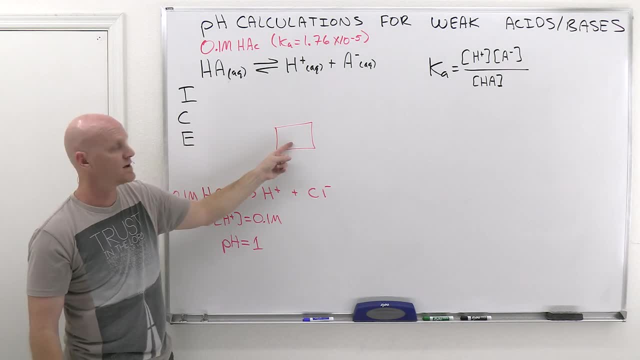 goes in that box right there The equilibrium concentration of H plus, And once I find whatever goes in that box that'll be the H plus concentration at equilibrium. I'll take the negative log to get the pH. So a little more of a process, much bigger pain in the butt. 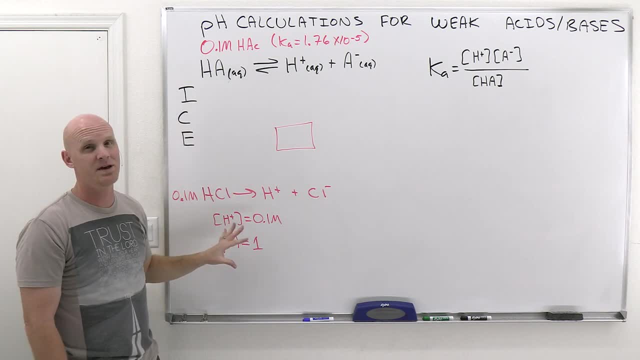 to find the pH of a weak acid as compared to the pH of a strong acid. However, once we do this the long way, once, I'm going to show you a shortcut as well, And we'll find out that, in the end, for most weak acids, there is a shortcut that's actually not too much longer than this. 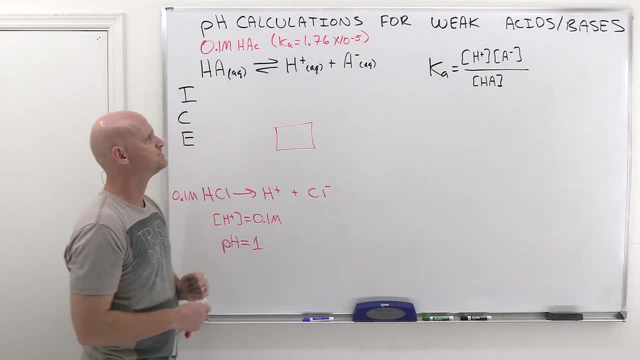 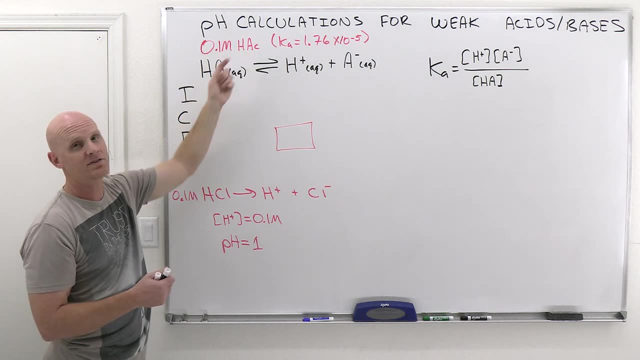 but it is a formula that you're probably gonna have to memorize, but we'll get there eventually, All right. So in this case, when we set up this ice chart, we're initially starting off with a 0.1 molar solution of acetic acid And again, 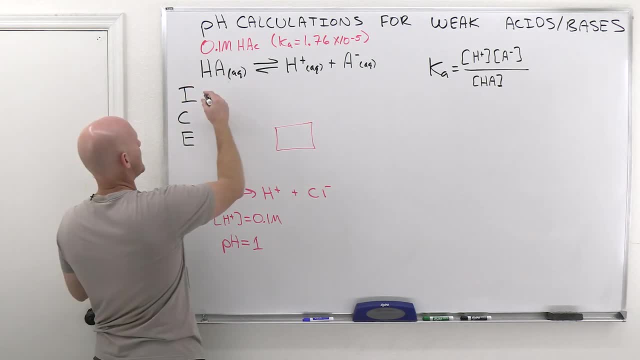 we can just use the generic reaction for any weak acid. So the initial concentration of the weak acid is 0.1. And before it dissociates you don't really have any H plus or any A minus. Now, technically, in pure water you do have a little bit of H plus 10 to the negative seven. 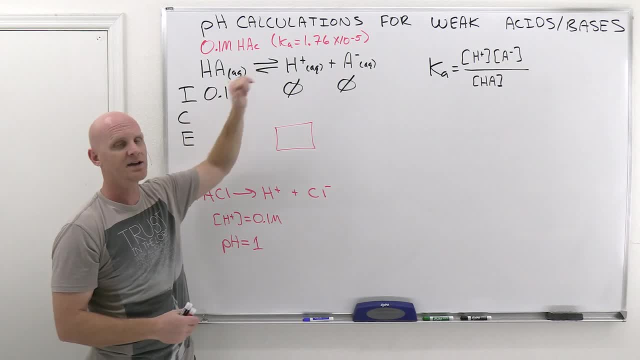 molar, but we're going to round that down to zero. It turns out that the amount of H plus we're going to get in this reaction is going to be much more significant than that. That's to the point where we can ignore that 10 to the negative seven molar, All right. Then the change when this dissociates: 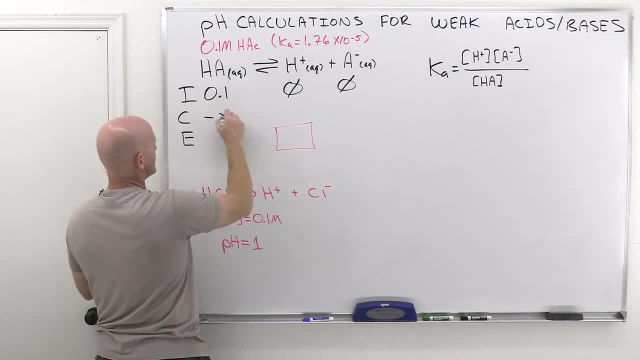 got to go right, because we only have reactants, we don't have any products. So we'll get minus X here, plus X here, plus X here 0.1 plus a negative X means at equilibrium we'll have 0.1. 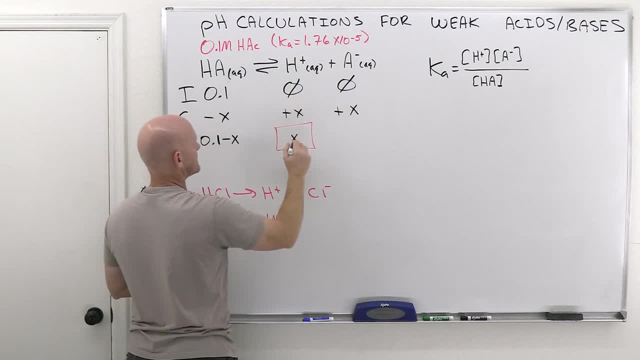 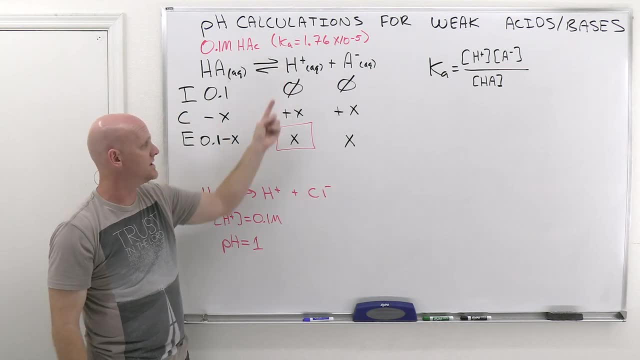 minus X: concentration zero plus X X concentration zero plus X X. And lo and behold, we're trying to solve for X, because X will equal the equilibrium concentration of H plus, And once we find that, we'll take the negative log to get the pH. but it's going to be a little bit. 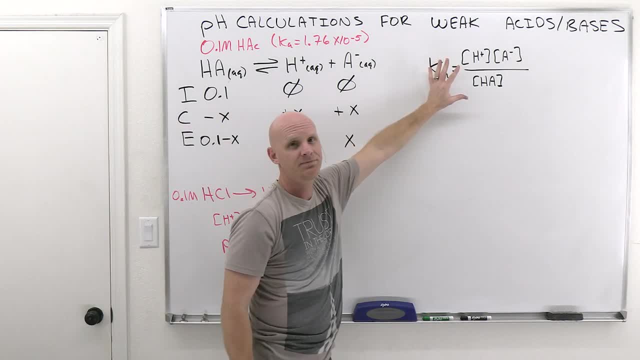 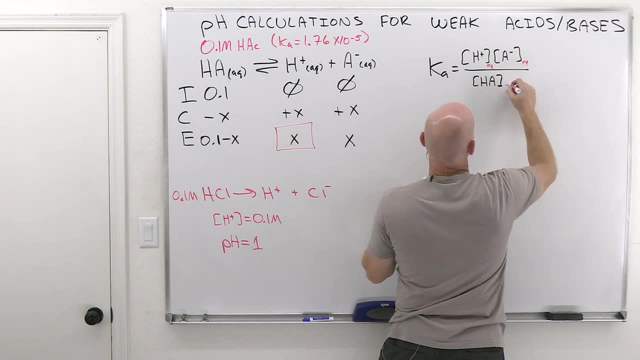 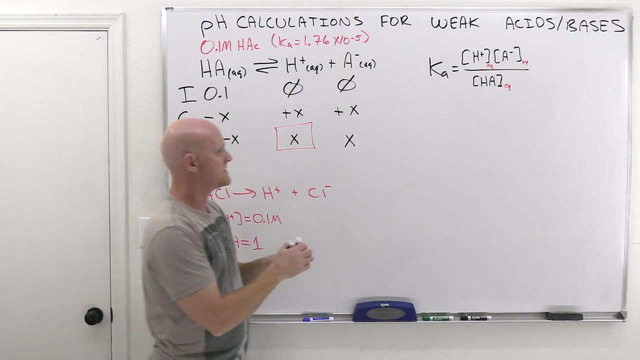 of a process here. So we've got our Ka expression and the Ka expression- don't forget that it's we don't usually write it, but it's implied that these are the concentrations at equilibrium, which is what are in these three spots on our ice table. And so, in this case, our Ka. 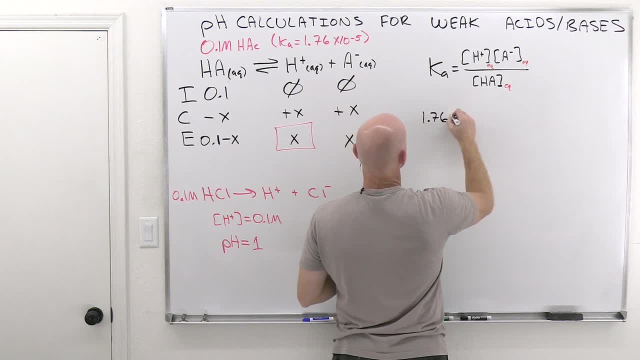 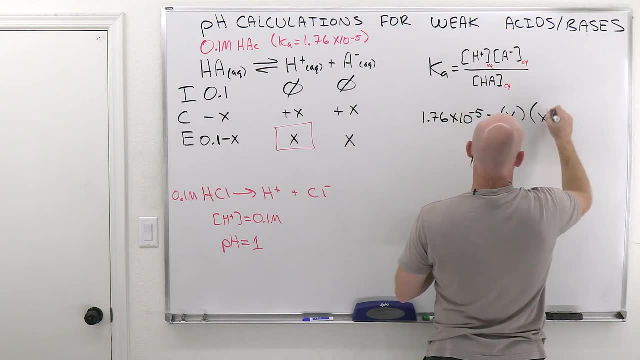 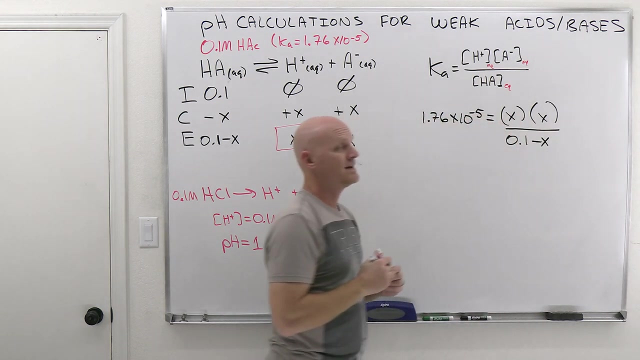 which was given as 1.76 times 10 to negative five, it's going to equal X times X, all over 0.1 minus X. Then we run into our first problem. If I asked you what is the most mathematically correct way of? 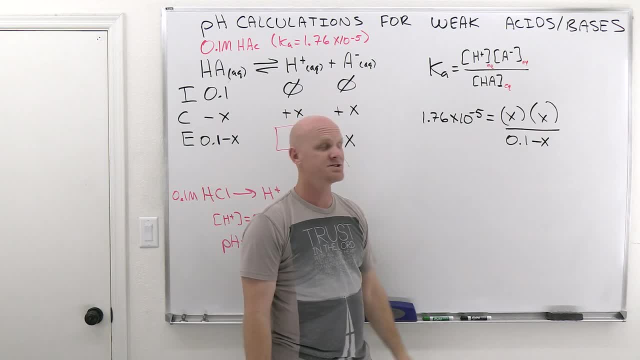 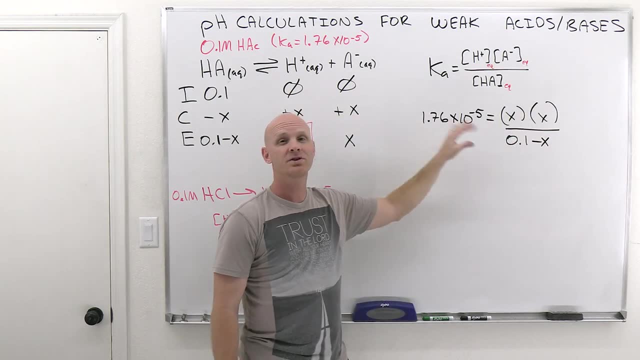 solving this. you should say the quadratic equation. You should multiply this 0.1 minus X up to the other side. This becomes an X times X, X squared, And then you should combine all the terms on one side, set up your quadratic equation to solve for X and it's going to suck Well. 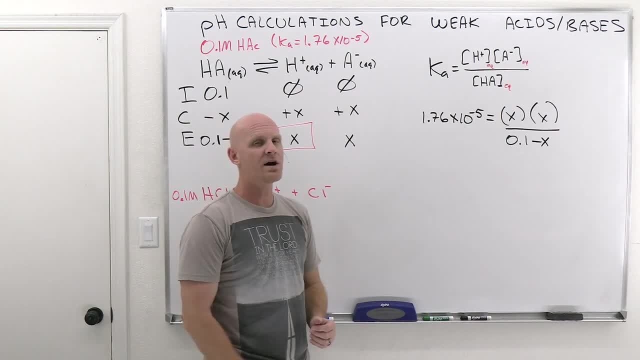 we're not going to do that, So we learned one way of getting around. the quadratic often occurs when you have very small equilibrium constant values. We learned this back in lesson 15.3.. And so in this case, that's exactly what we have. All your Ka's you're going to deal with are going. 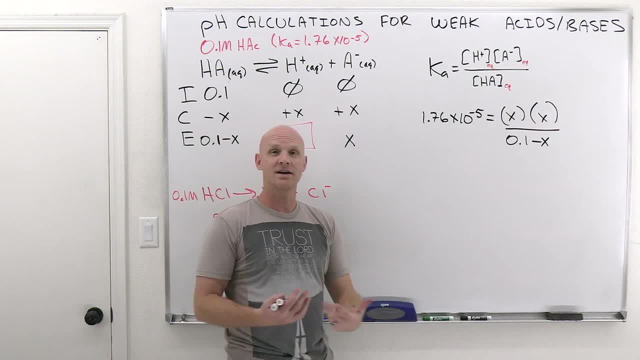 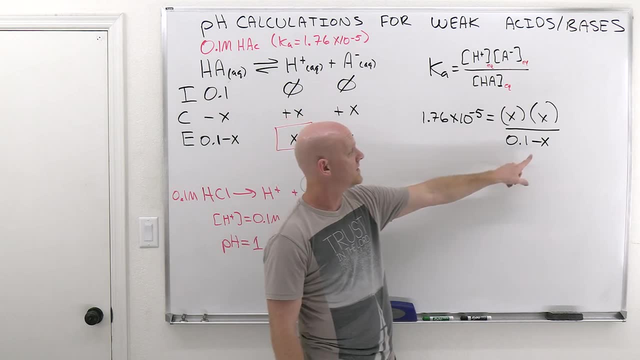 to be small values, because weak acids typically dissociate less than 5%. So life is good in that respect And in fact, as long as they're dissociating less than 5%, we're going to get to ignore that little minus X in the bottom, like we did in one of the examples. 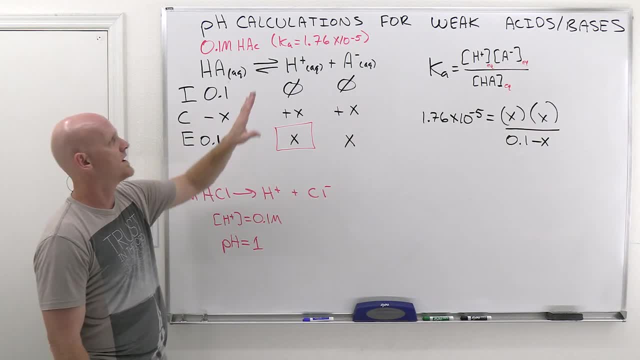 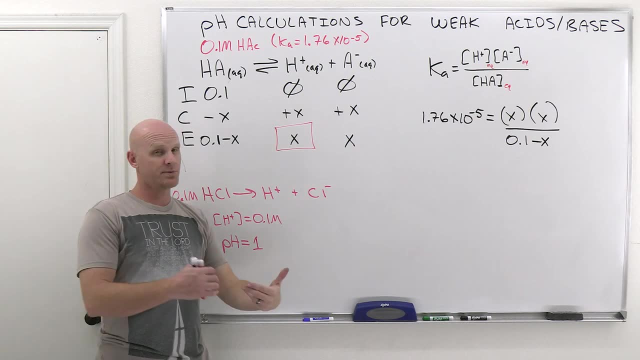 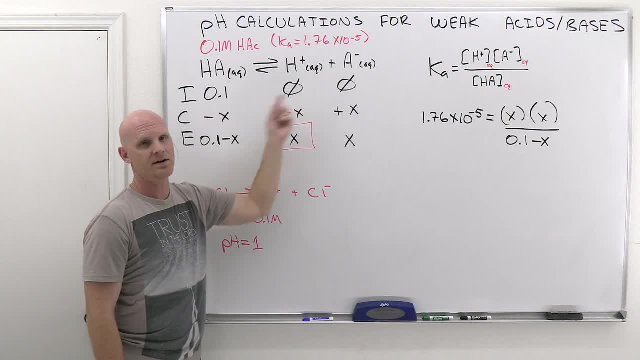 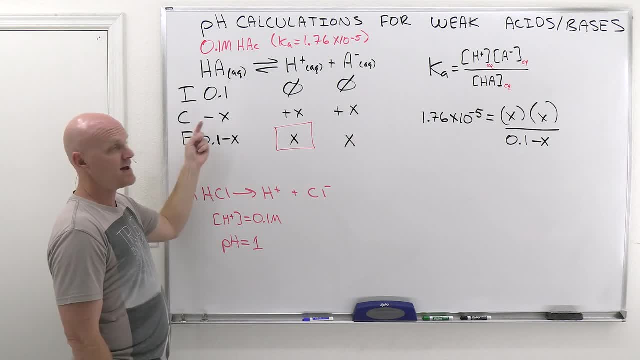 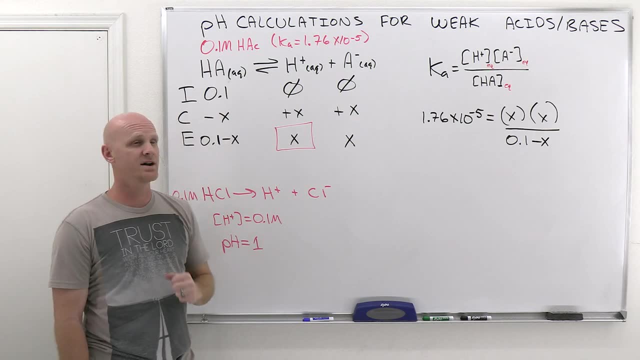 mostly only reactants, which means that the amount that reacts X here is going to be small, And so a small equilibrium constant is going to be the key for us to realize that we should have a small value of X. Now, this X times X, when you multiply by a small value, it changes things. It. 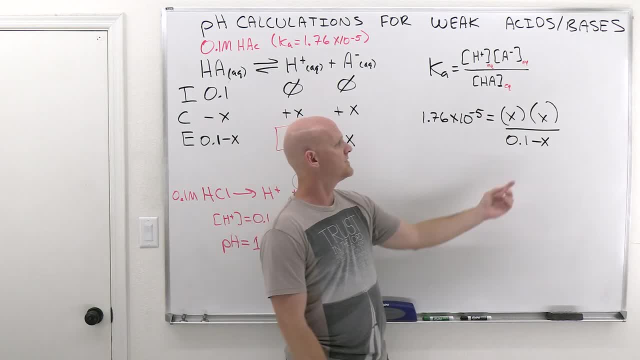 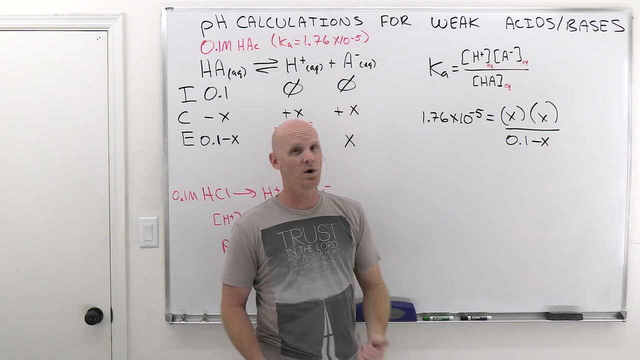 has like a very significant impact on the equation. The key is when you add or subtract a small number- 0.1 minus a really small number is, for all practical purposes, still 0.1. And how small is small enough to ignore? Well, if the number you're subtracting is less than 5% of what you're. 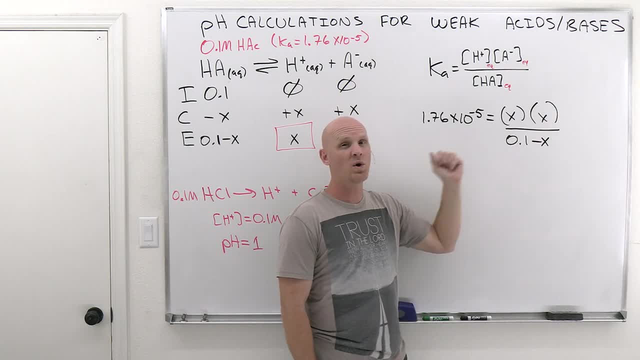 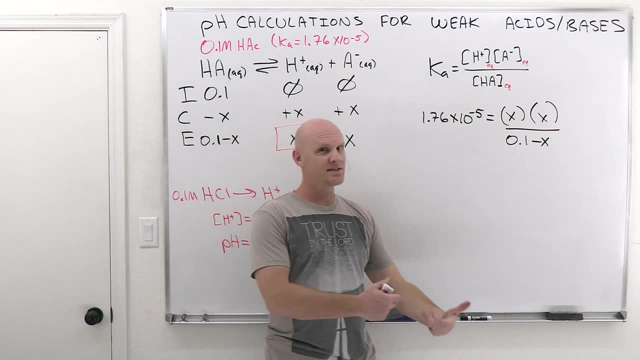 subtracting it from. if X ends up being less than 5% of 0.1, then ignoring it will make very little difference on the equation And since most weak acids do dissociate less than 5%, that'll typically be the case. Now, if you get one that's associating more than 5%, then you really should use the. 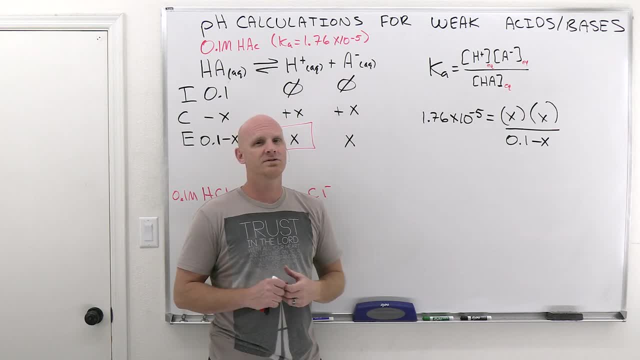 quadratic. Now here's the deal. Most weak acids do dissociate less than 5%. Now if you get one that's associating less than 5%, then you really should use the quadratic. Now here's the deal. Most of you are going to be told one of two things: You're either going to be told you're never. 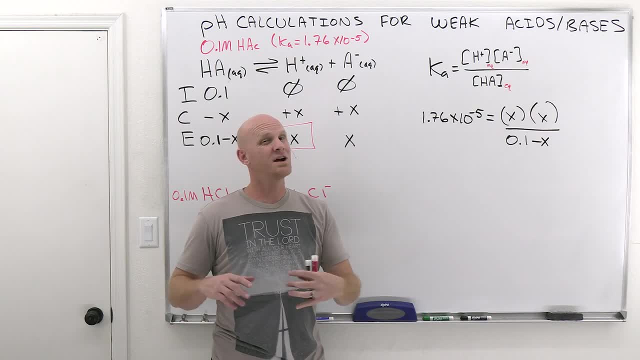 going to have to use the quadratic, or you're going to be told that it might show up on the homework, but you're never going to have to use the quadratic on the test because it just takes too long. So, and for those of you that are still on the hook for the quadratic, I apologize. The 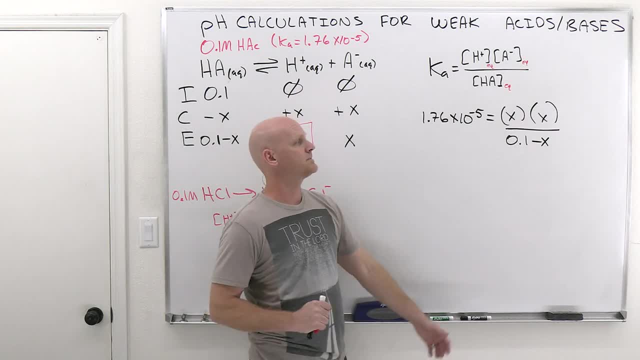 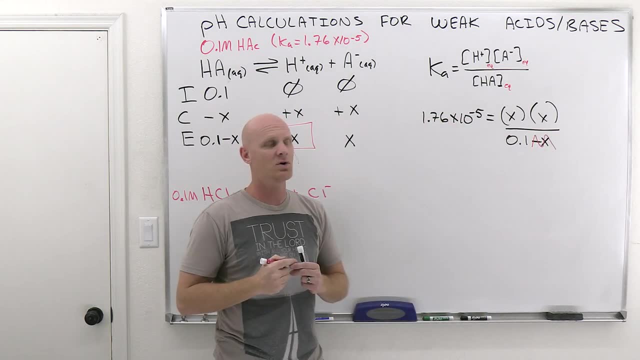 shortcut we're going to learn may not always apply to you. So, however, in this case, though, I'm just going to blanket assumption that this minus X is going to be statistically or mathematically insignificant: It's going to be less than 5% of 0.1 and won't have minus X. 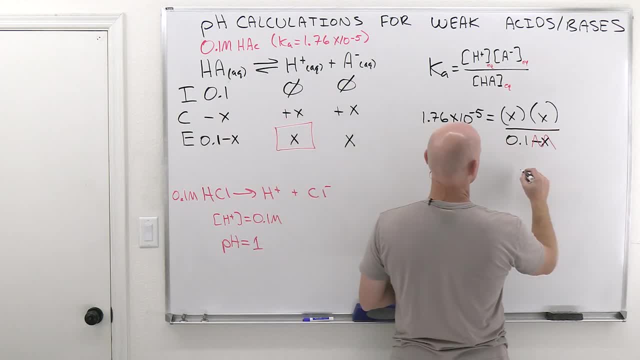 So ultimately this is going to turn into: X squared over 0.1 equals 1.76 times 10 to the negative 5.. And then I'll multiply this side up by 0.1 and let's make that look a little more. 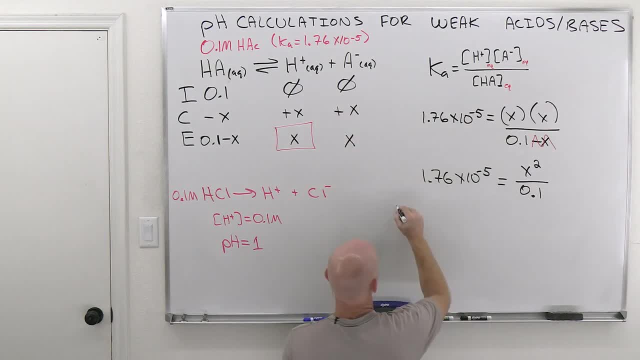 like a decimal point, And so we're going to get 1.76 times 10 to the negative. 5 times 0.1 equals X squared, And then just solve for X from here. We're just going to take the square root. 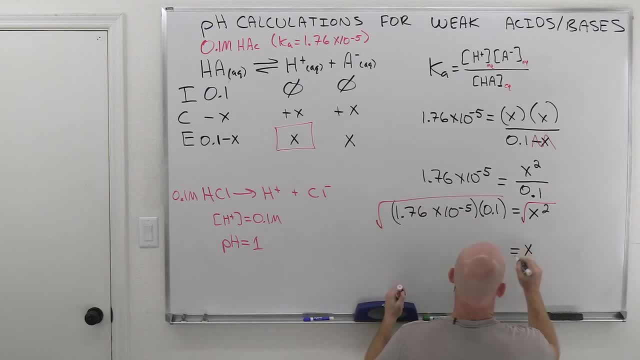 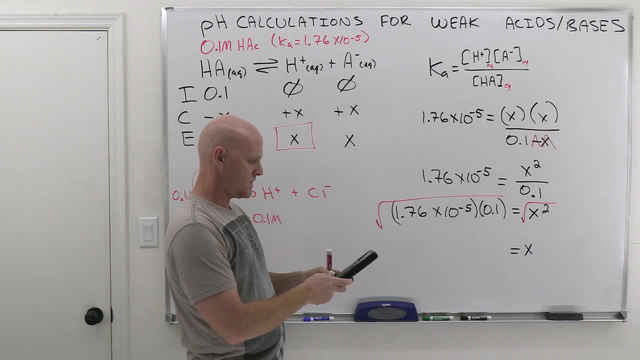 of both sides and definitely going to take advantage of our calculator right here. So in this case I'm going to take 1.76, 10 to the negative, 5 times 0.1,, which is 1.76 times 10 to the negative 6.. You might've been able to do that in your head. 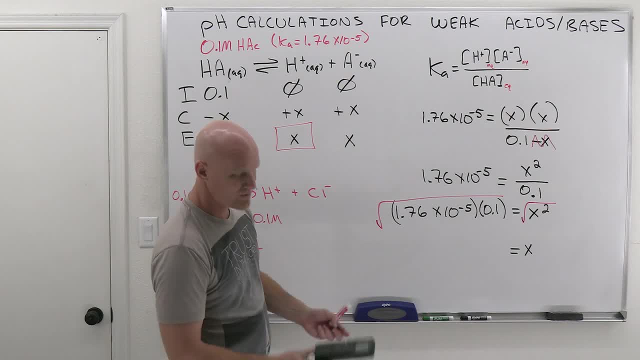 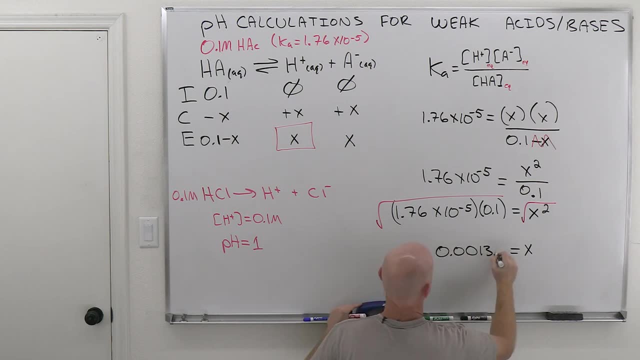 And then we'll take the square root of that and get 0.0013, rounded to two sig figs here. So we're going to take 0.0013, rounded to two sig figs here- Cool. And if you recall our whole goal, we've been a long ways through this process. 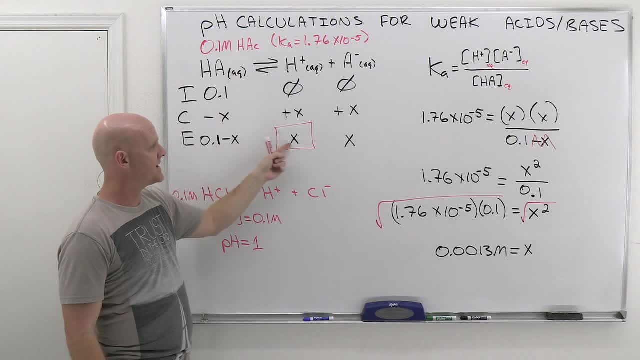 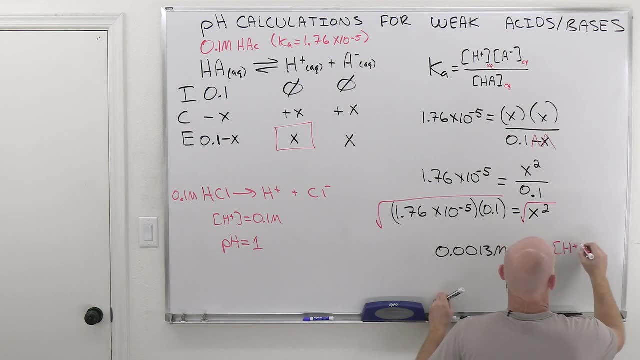 but our whole goal again was to find this equilibrium concentration of H plus, which just happens to equal this X value. So this is the H plus concentration, So, and in fact it's also the A minus concentration. And if you want to figure, 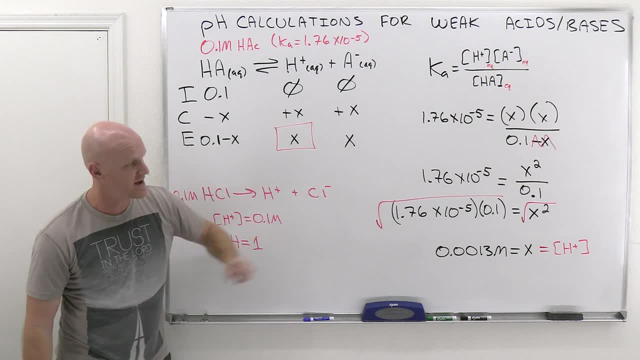 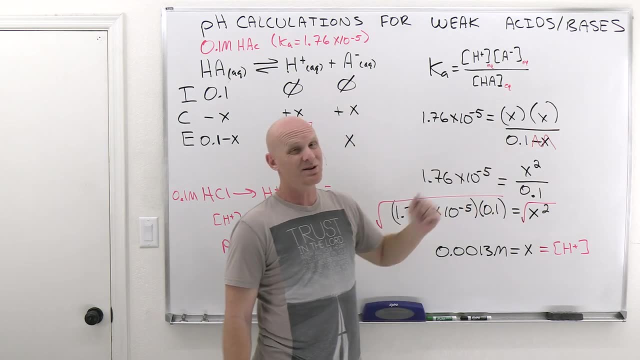 out what the exact HA concentration is. well, it's 0.1 minus that number, which is pretty close to 0.1.. So 0.1 minus that small number is, for all practical purposes, still pretty close to 0.1.. 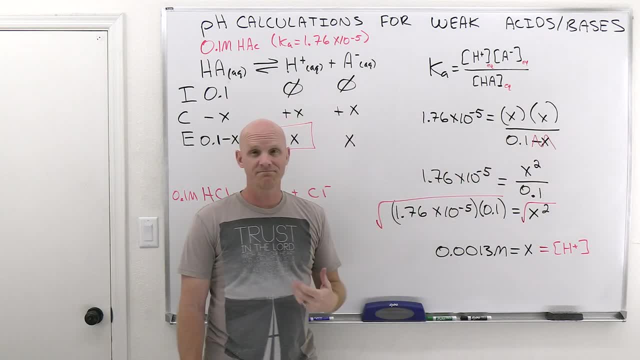 So in fact, again, as long as X was less than 5% of 0.1, ignoring it here in this case is a good idea. And in fact, if you take 0.0013 and divide it by 0.1 and times a hundred, you'll find out. 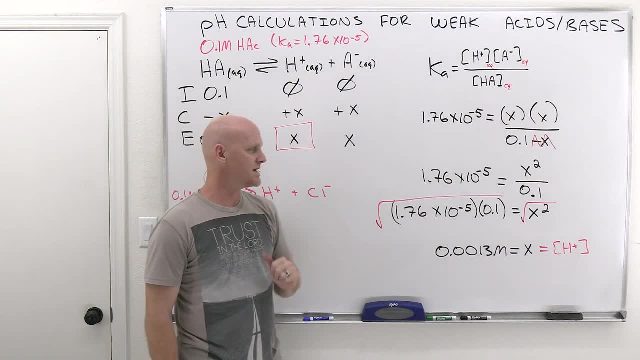 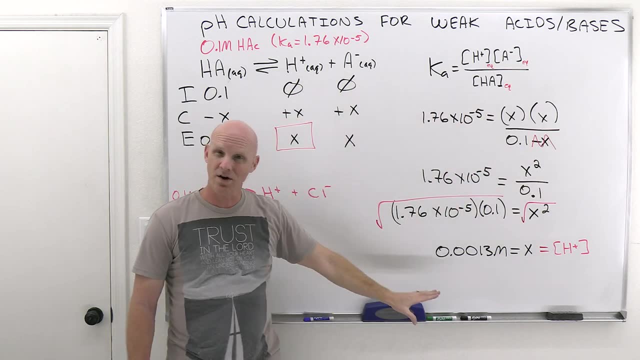 that it's just 1.3%, definitely less than 5%, And so, whether you ignored this, like we did, or whether you didn't ignore it and set up a quadratic and solved it, you get roughly- I shouldn't say roughly. you get really close to the exact same answer either. 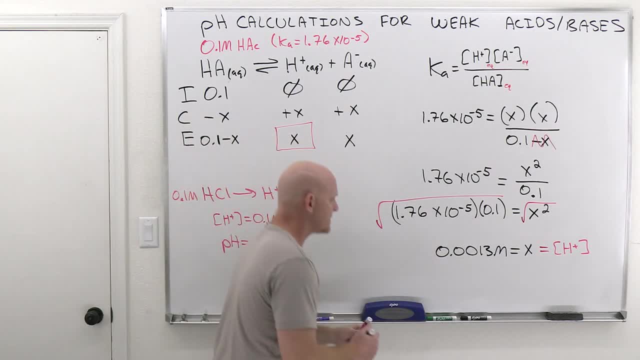 All right, And since that's your H plus concentration, we'll just take the negative log of this. And the negative log of my last answer in my calculator is going to be 2.88 or 2.9.. I'll round it to 2.9.. 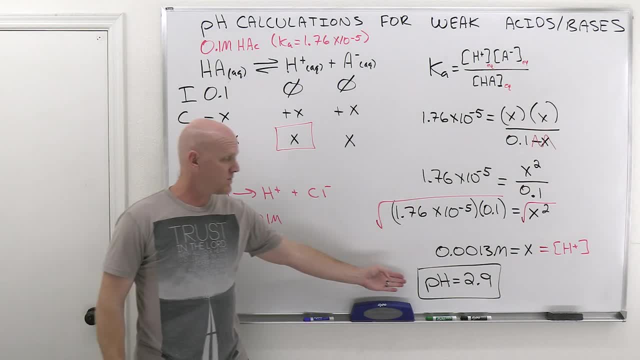 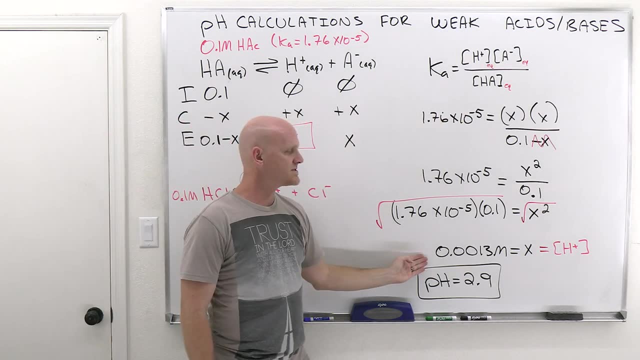 Cool. A lot of work to come out with a pH for a weak acid here. Ice table- creative way to avoid the quadratic and then finally solve for X and take the negative log and get the pH. So this is the process. You should know how to write. 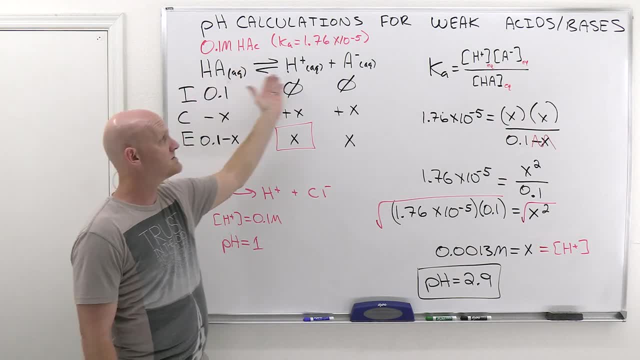 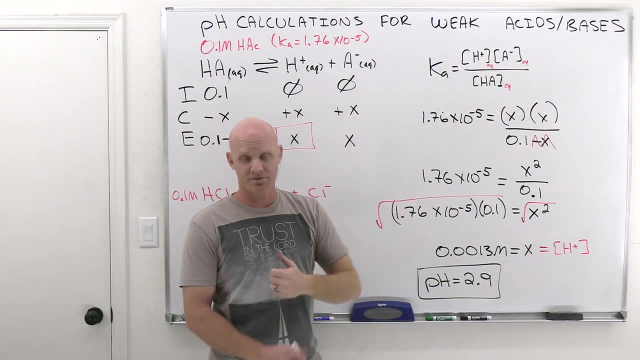 generically this expression. You should be able to write the reaction for any specific weak acid as well. You should be able to set up a generic Ka expression or a specific one for any weak acid as well, But as far as the calculations go, 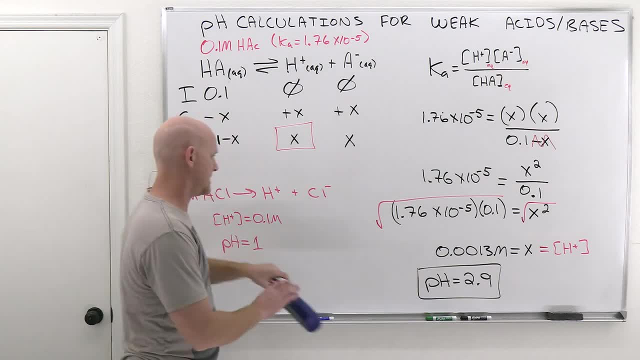 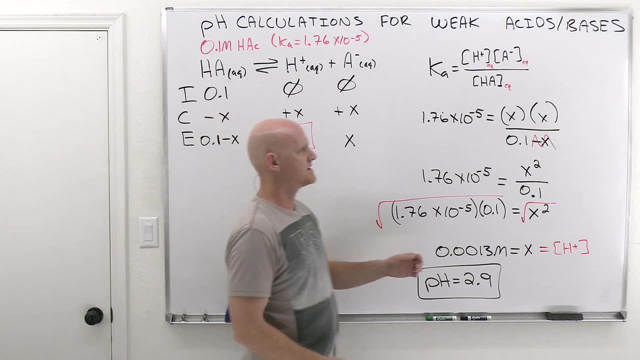 here's what you can take away for a shortcut here. So it all comes down to this step, right here. So because, again, assuming it dissociates less than 5% and that you're going to avoid the quadratic, either because you're told you're never going to have to use the quadratic or, in most, 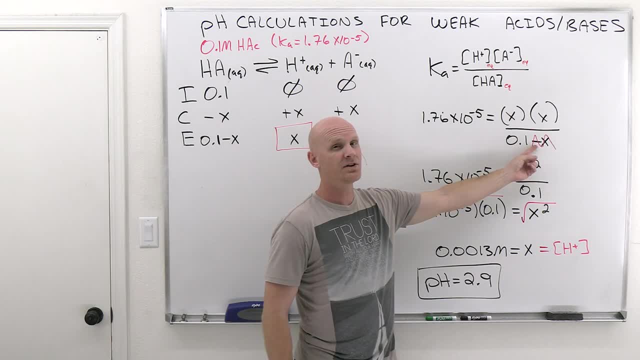 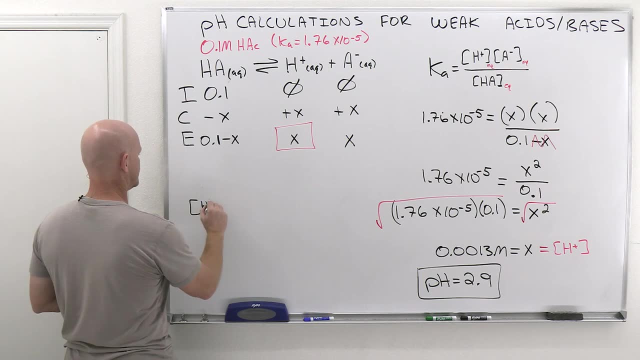 cases it's going to be less than 5%. anyways, we're just going to blanket assumption. ignore that minus X right there and take a look at what falls out here. So in this case, X happens to be your H plus concentration. So when we solve for X, it was equal to the square root of our Ka value. 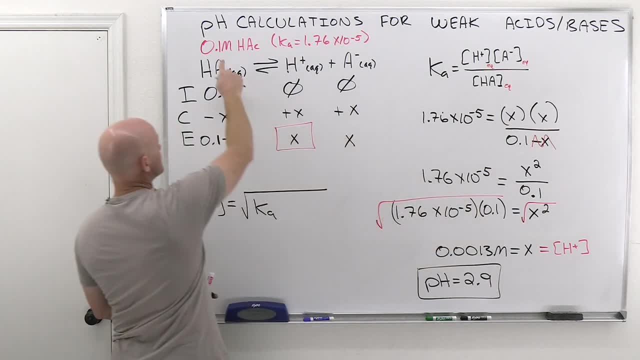 times the concentration, the initial concentration of the acid, And the idea it really should be the equilibrium concentration that we plug in there. But again, as long as the minus X is statistically insignificant, well then, approximating the equilibrium value as the same as the initial value. 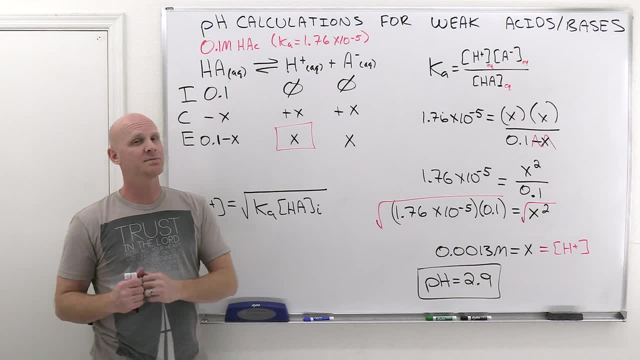 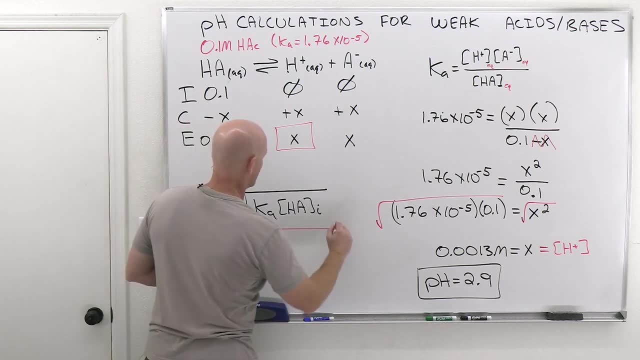 they're going to be really close, because the amount that associated was typically going to be less than 5%. So that's kind of the deal here. So this is what this ultimately turns into, And for any weak acid, you can pretty quickly calculate the H plus concentration and then take the negative logging. 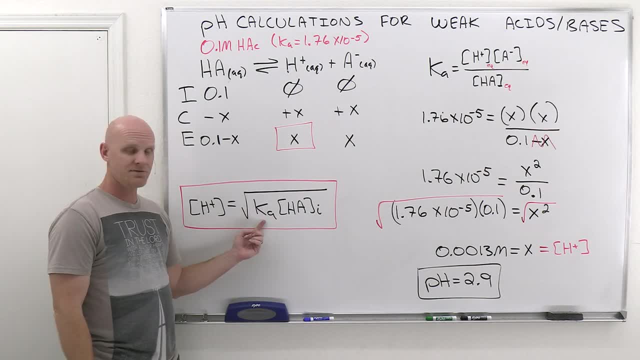 to the pH. You've got to be told two things though: You need to know the Ka for the acid and the acid's concentration. But assuming you're provided with those too, you just multiply them together. take the square root, That gets you the H plus concentration, And then you 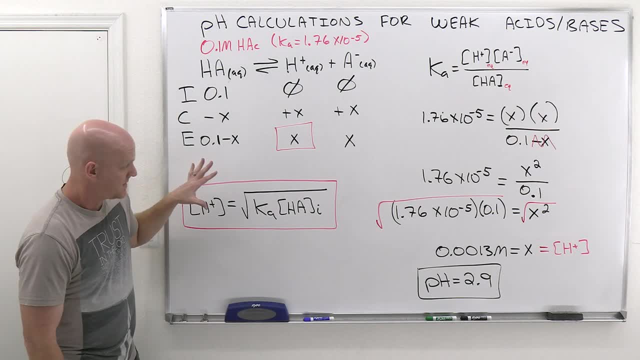 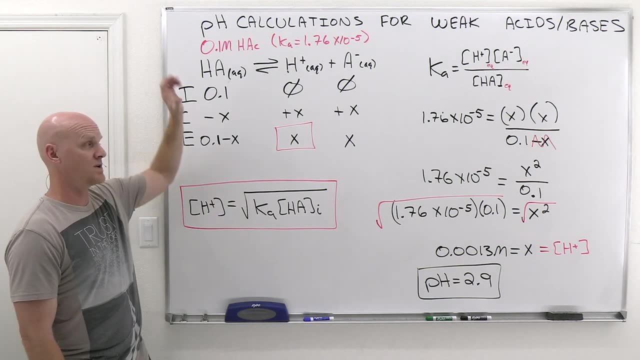 take the negative log And that's it, And so typically you're not going to be given this little shortcut. So it's something you might have to memorize but worth your time to memorize, because we can avoid an ice table and the shape of the pie, But then you never really want to make. 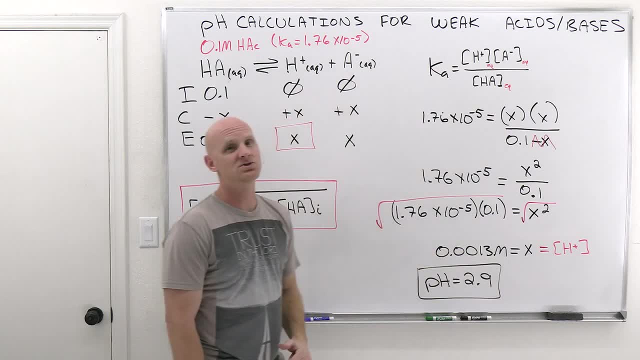 like that, shottoes and transformer. what do you do? Well, you try to cross out least two. maybe you can easily ơi that. And if you get an equation where less than 4% but less than 5%, and this lovely calculation and things of this sort and make it really quickly something that's. 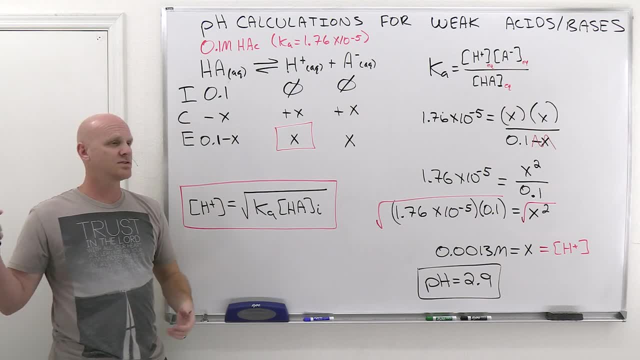 only a little bit slower than solving for the pH of a strong acid- Strong acid dissociated completely- we could get the H plus really easy and then take the negative log. Well, now we have a little bit harder method- but not bad- of way of getting the H plus concentration. 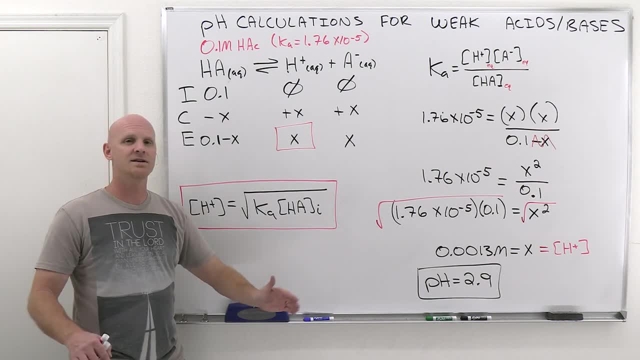 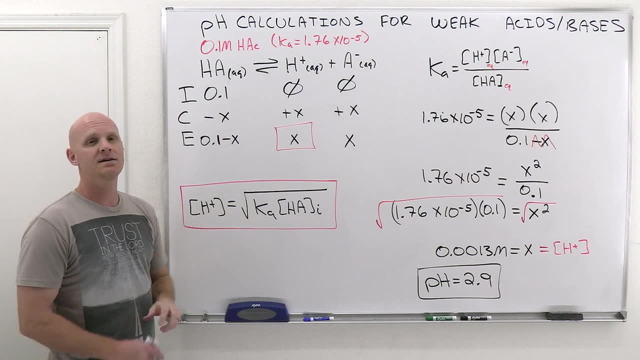 of a weak acid, Ka times Ha square root, and then take the negative log and we're done. So not so bad for a weak acid once you get here. So let's keep this in mind as we take a look at the next problem. Okay, so if you're being asked for the pH of a weak acid, we now know a. 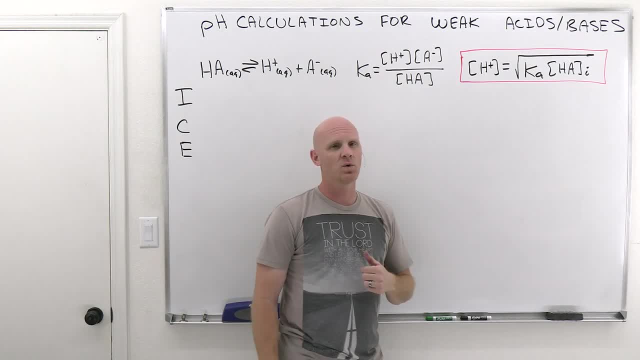 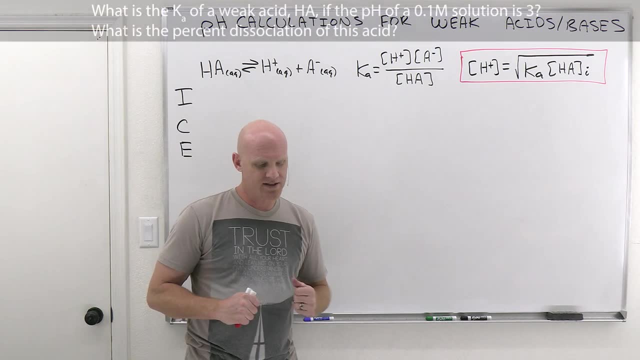 really good shortcut that will work most of the time- well over 90% of the time for most of you, if not 100% of the time. But what if the question is not what is the pH, or something like that? So like this next one says: what is the Ka of a weak acid? Ha, if the pH of a 0.1 molar solution is? 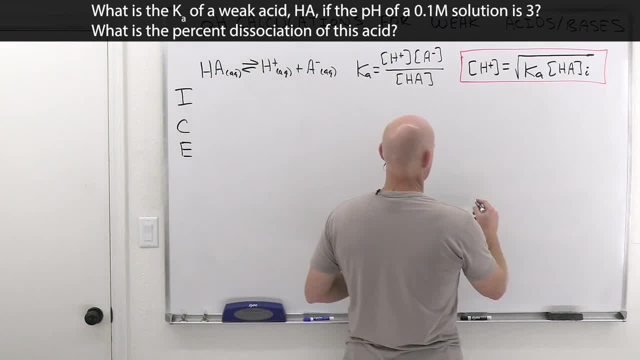 three. So this time we're given the pH, And so the idea is that the pH equals three. And the big thing you're supposed to realize here is that, well, if the pH of a weak acid is three, then the pH is three. Well, that means the H plus concentration is 10 to the negative three molar. 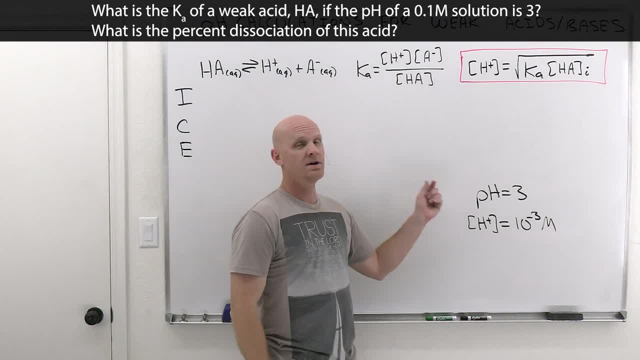 same as one times 10 to the negative three molar. You might recall that we learned when you know the H plus concentration, the pH, the OH minus concentration or the pOH. if you know any one of those four, you can calculate the other three. So by giving us the pH, what they really gave us. 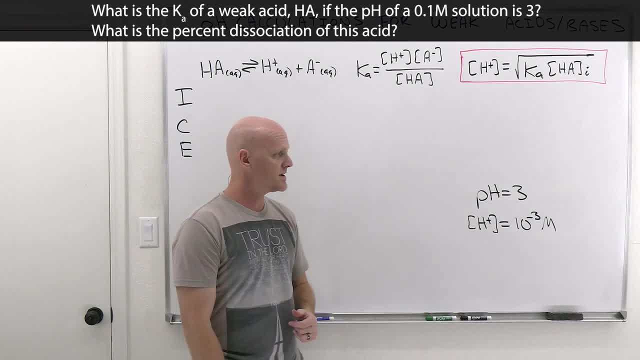 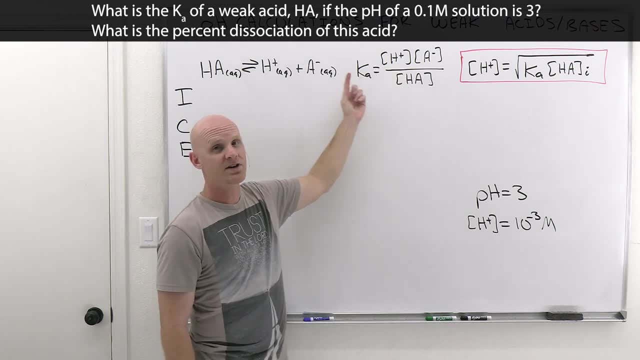 was the equilibrium concentration of H plus a way of knowing that equilibrium concentration. So that'll be key. And so in this case we know the equilibrium concentration of H plus is 10 to the negative three molar And we're being asked for the Ka Well. 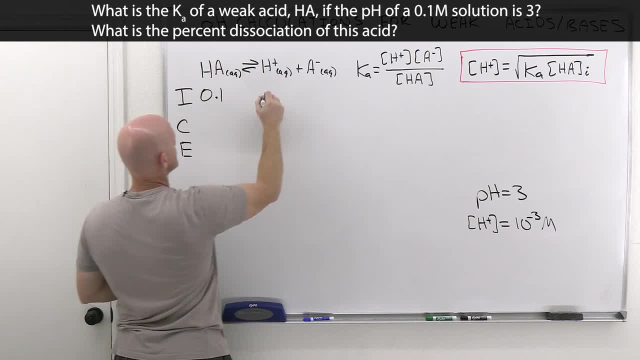 if we set that up, it's a little easy to do, But let's just keep in mind. you know, once we set this up before with a 0.1 molar solution of a weak acid, we set up that whole ice chart a little bit ago. 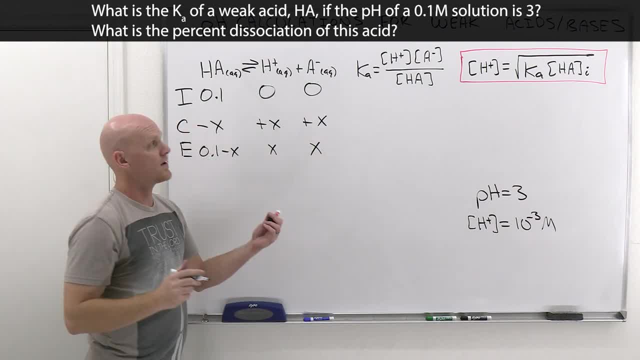 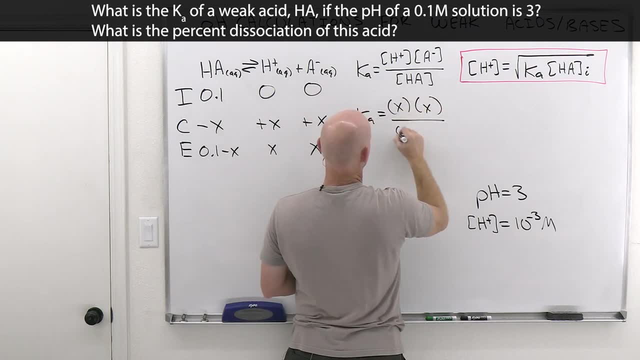 and it looks something like this: 0.1 plus negative x was 0.1 minus x, 0 plus x was x, 0 plus x was x, And so the result of our ice table is that our Ka value is going to equal x times x all over 0.1. 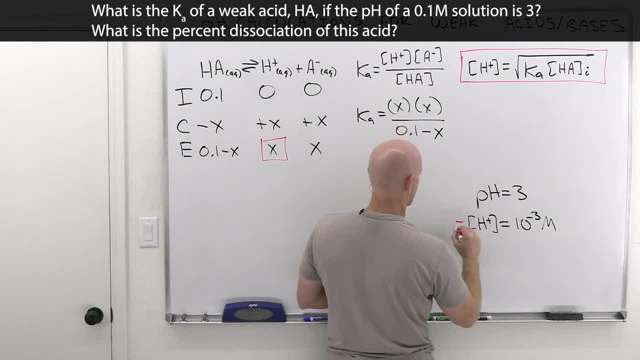 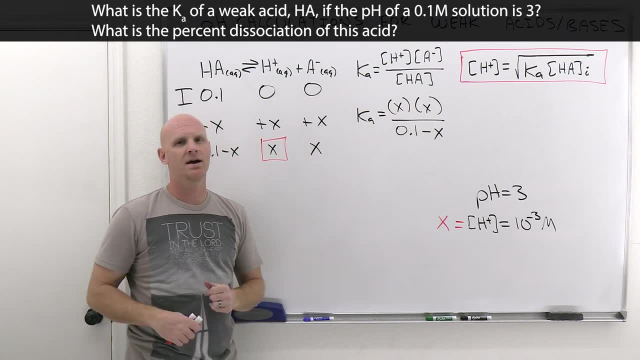 minus x: 0.1.. 0.1. 0.1.. three molar, which just happens to equal X. Well, if equals X, then by all means just plug it in and you can solve for KA And you might be inclined. well, Chad, you just ignored the minus. 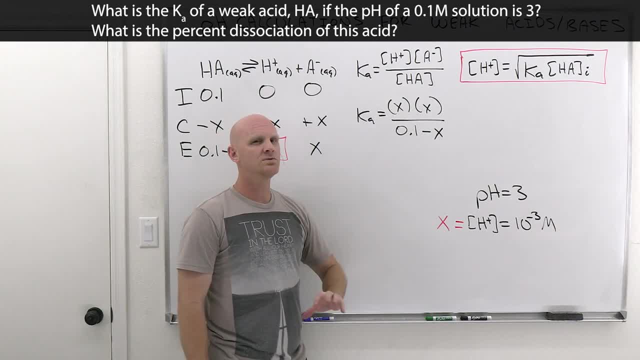 X. right, Well, you can. but the whole reason we did that in the last problem is because we were solving for X And in solving for X. if we don't ignore that, it sucks. It's a quadratic, But in. 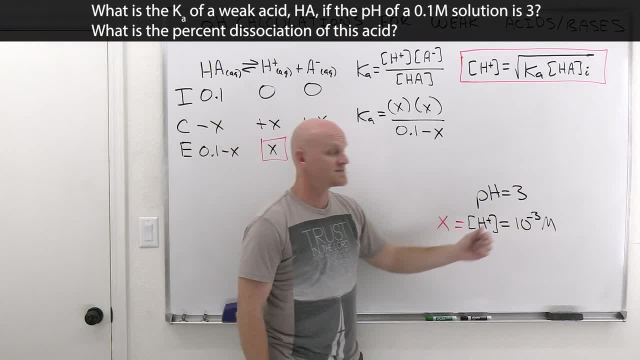 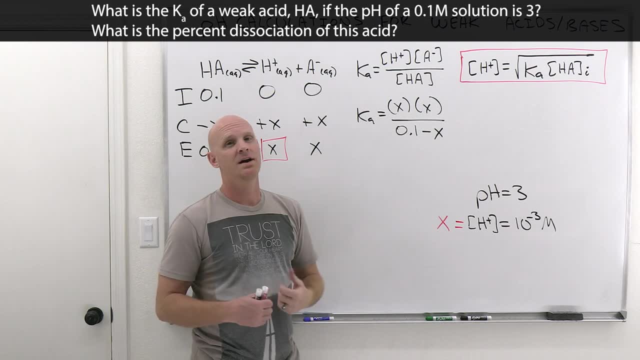 this case, we're not solving for X, we're solving for KA, and we're just substituting this in for X, And so the truth is there's no quadratic here, regardless of how you solve it, So you might as well get the best and most accurate answer by including it there, But the truth is you're. 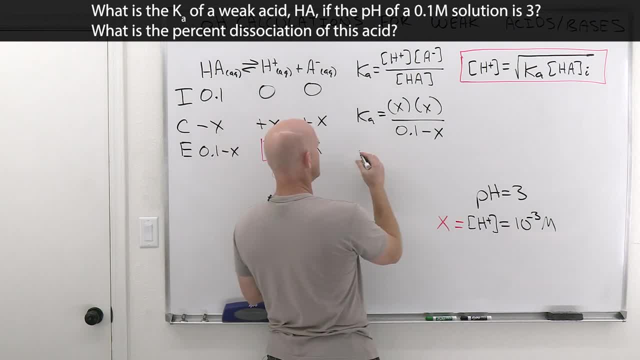 right, it probably isn't going to make a difference. But since we're not solving for X, it doesn't matter. We're not going to have to solve a quadratic either way. So in this case, X squared would be 10 to the negative 3 squared on top, all over 0.1 minus 10 to the negative 3.. And that's. 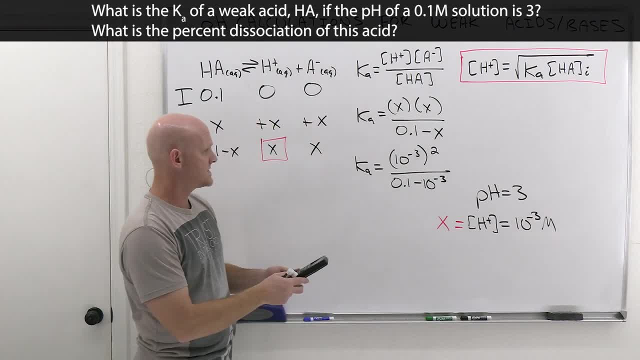 our KA value. So let's take a look here. So 1 times 10 to the negative 3, so I'm plugging that into my calculator and I will square that and then I will divide that by 0.1,. oh, let's get my parentheses in there. 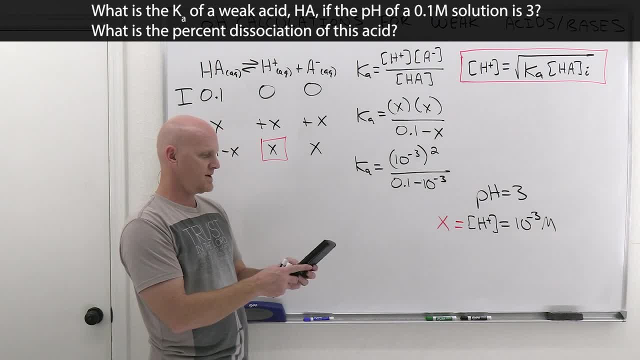 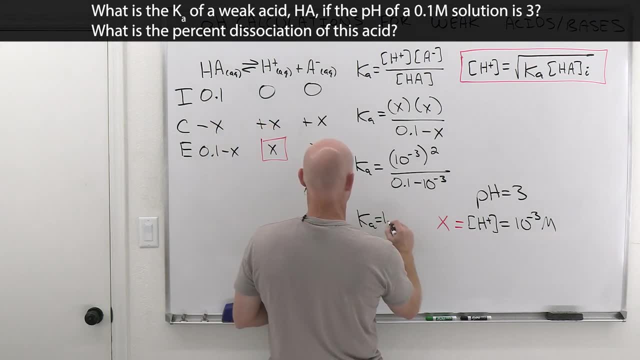 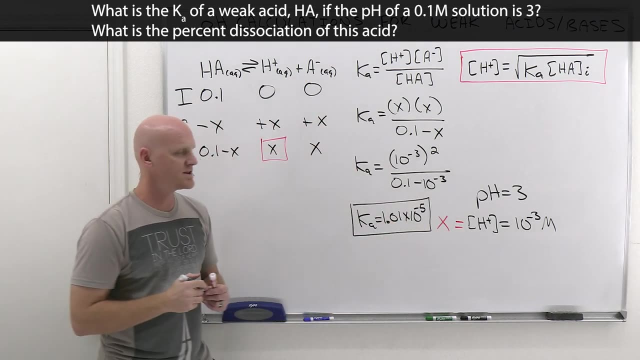 0.1 minus 1 times 10 to the negative 3. And I'm going to get 1.01 times 10 to the negative 5.. That is our KA value. That's the first half of the question here. 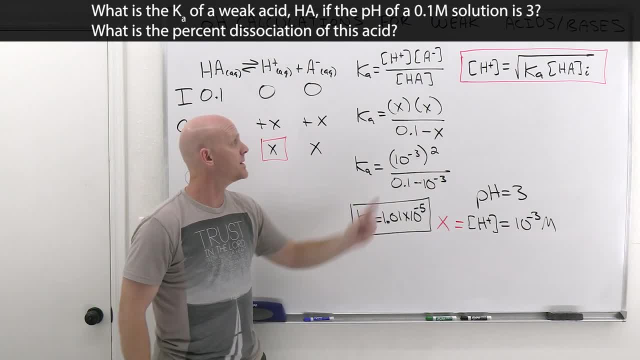 How do you solve for X? Why did you ignore this right here? this minus 10 to the negative 3?? The minus X? if you will, then you would have just got 1.00 times 10 to the negative 5, and you're right, it really didn't. 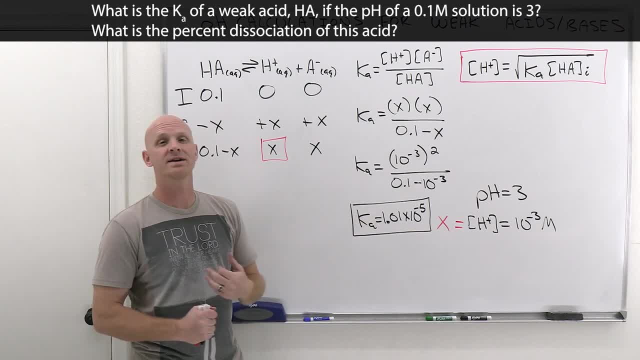 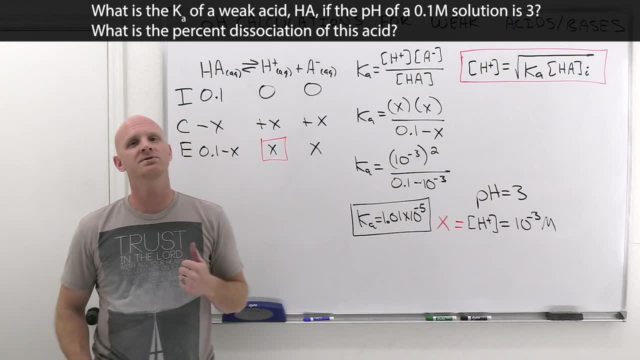 make much of a difference. I always just cover my bases in getting a slightly more accurate answer, just in case they gave you an example where it did make a difference. Second half of this question says what is the percent dissociation of this acid. So what percent did it dissociate? Well, 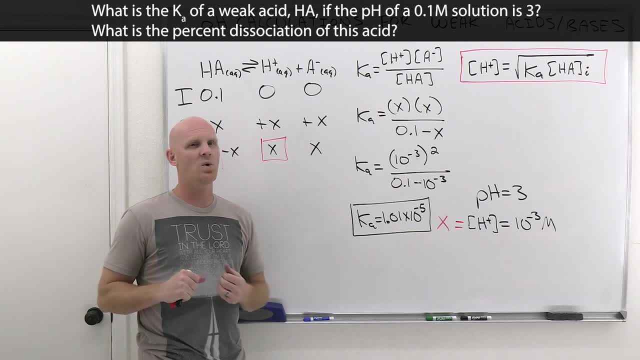 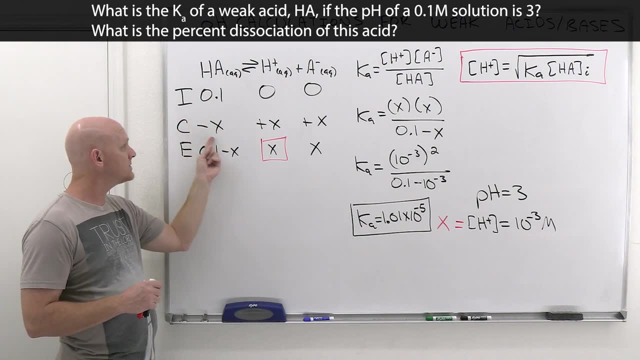 probably less than 5%, but what exact percent? And this is another way this question could be asked. Well, if you look, the amount that dissociates is X. You start off with a certain amount, but then you lose a certain amount. Why? 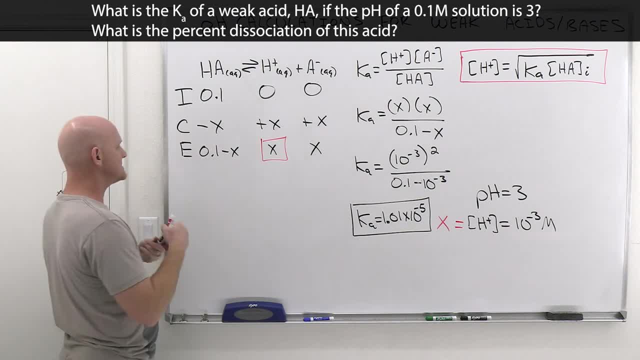 do you lose some Because it dissociates, And so X is the amount that dissociates. And so if you want to get the percent dissociation, you take the amount that dissociates divided by the total amount that you started with, and then times 100. And so it's X from. 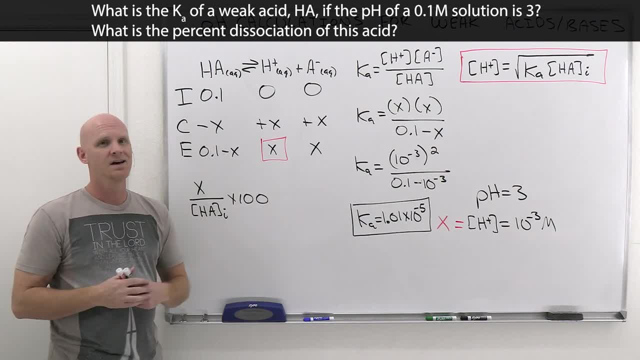 the ICE chart over the initial acid concentration times 100.. That's percent dissociation. Well, because X is typically equal to the equilibrium concentration of H plus, you'll see people write it this way instead because it's so common to know the H plus. 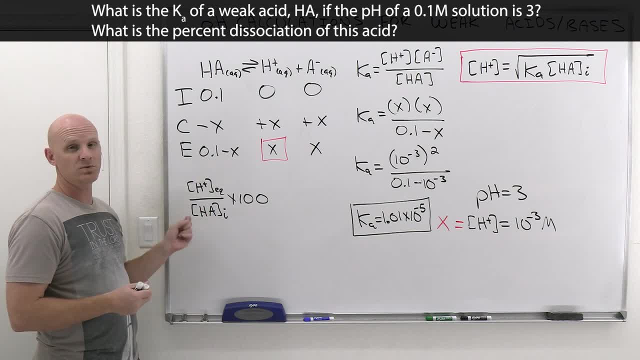 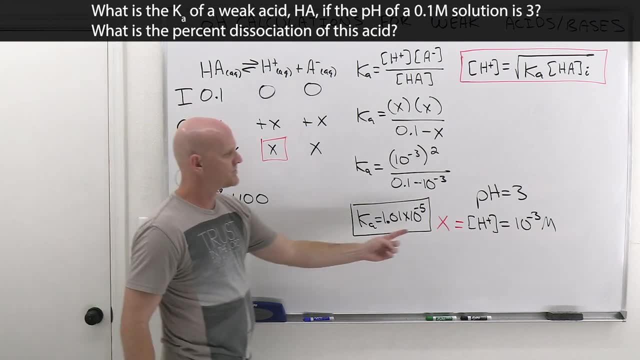 concentration, or have found it, And so in this case you could look at it this way as well: Instead of X, which just happens to equal the equilibrium concentration of H plus, you can do this calculation as well, And so we already knew the H plus concentration was. 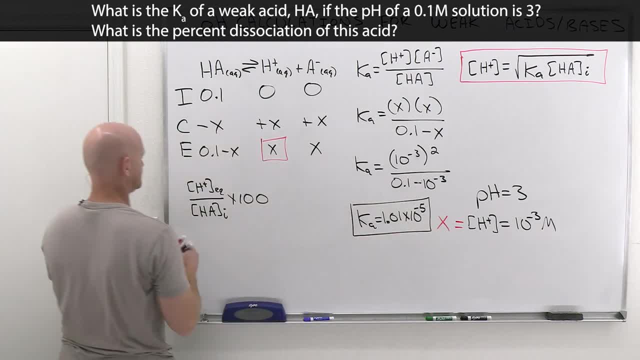 10 to the negative 3 molar, which was X, And then the initial HA concentration was given as 0.1 molar essere 100 times 100, and we'll find out that this equals one percent dissociation. So cool. And then examples of all. 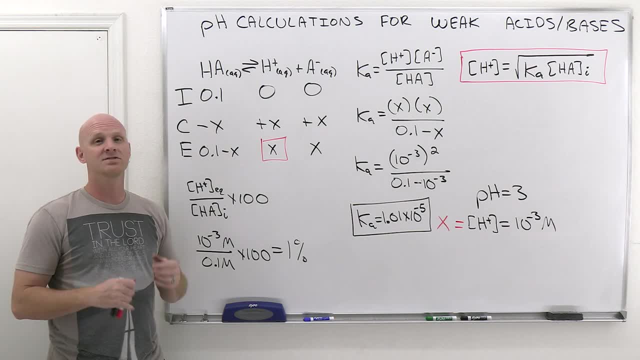 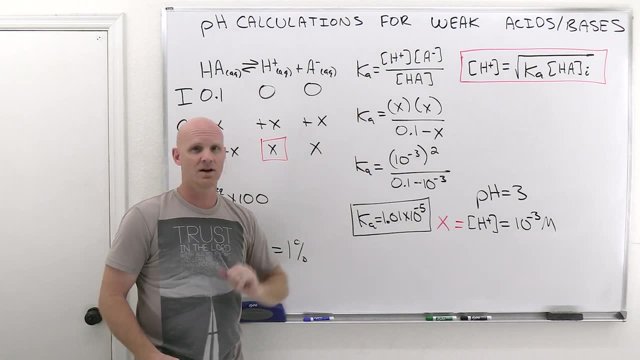 three types of calculations you might find for a weak acid And again, the most common is definitely finding the pH, which we did in the first example. Or you might be given the pH and asked to solve for Ka, which is what we did in the second example. Or you might be asked to solve for 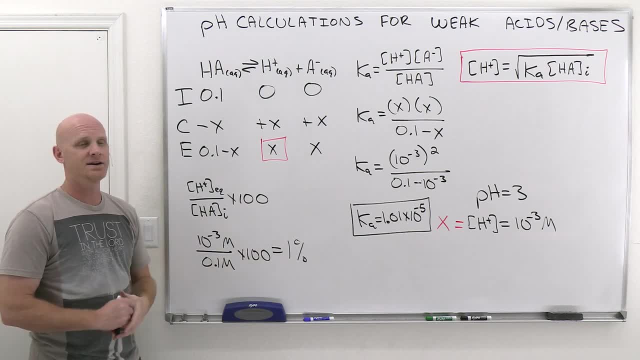 the percent dissociation, which we did right here. Cool. These are weak acids. We'll do this pretty analogously for weak bases as well. Let's dive in, All right. so we're going to take a look at weak bases and I'm going to kind of cut to the chase here and skip to the end for just a second. 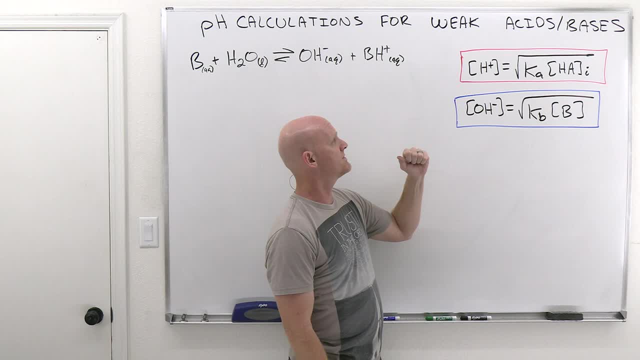 We found out with weak acids that we could actually summarize. you know very quickly how to find the H plus concentration with a little shortcut that works well over 90% of the time for most weak acids- typical when they're dissociating less than 5%- We just take the. 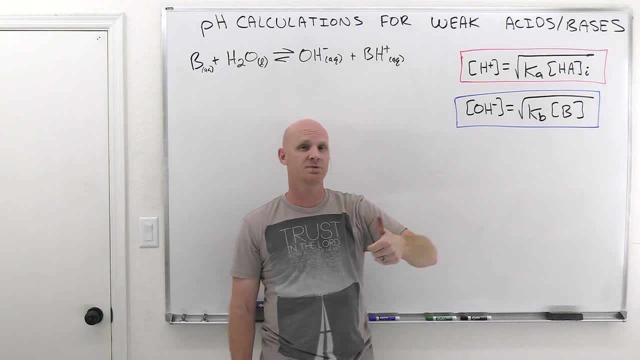 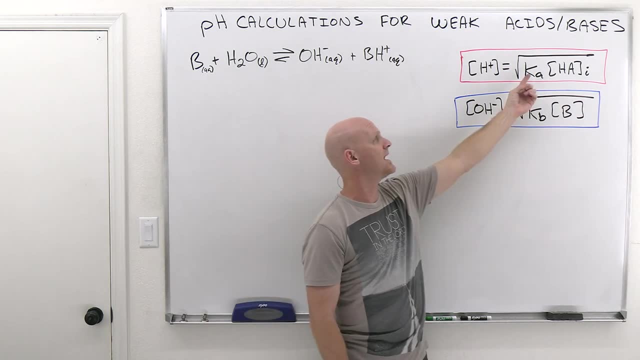 Ka times the initial concentration. multiply them together. take the square root, you got the H plus. take the negative log, get your pH. Well, it turns out. there's an analogous expression that we're going to derive here in a little bit for a weak base Instead of a Ka, though we're going. 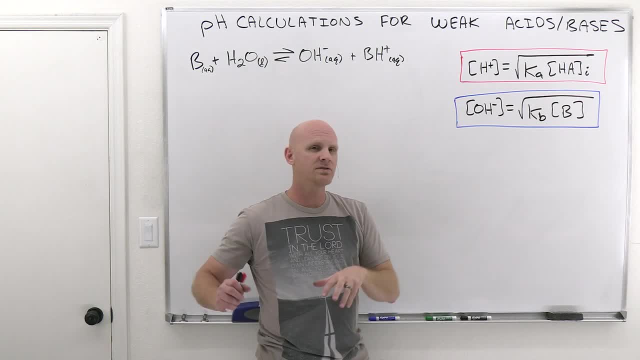 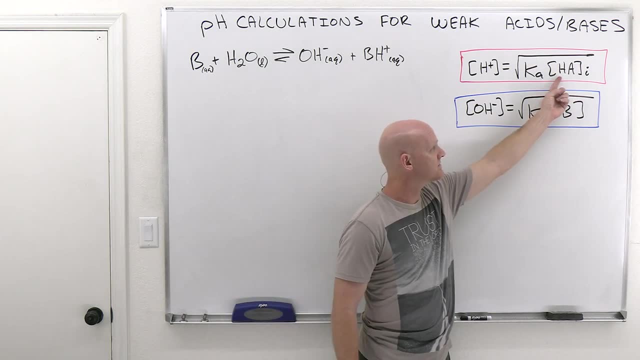 to find out. you have a Kb for bases instead. So for a weak acid dissociating water, the equilibrium constant is called Ka. For a weak base dissociating water, it's called Kb. And then, instead of the acid concentration, you're going to multiply by the base concentration. And when you multiply, 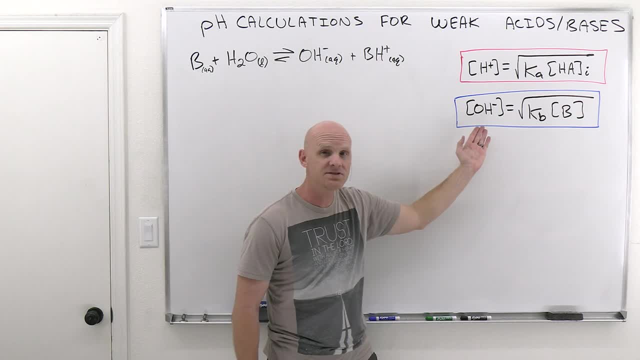 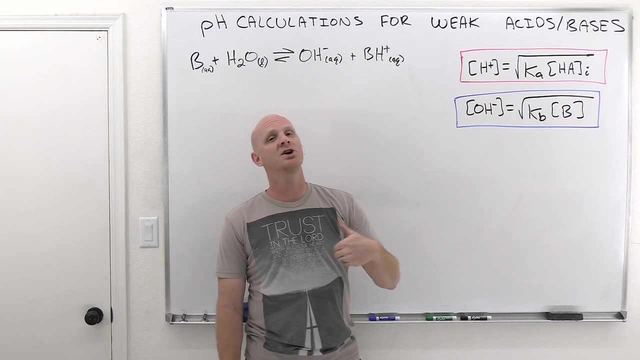 them together and take the square root. well, for an acid you get the H plus, but for a base you're actually solving for the hydroxide concentration, And so when you take the negative log, you're not going to get the pH, You're going to get the pOH, and then you'll have to subtract. 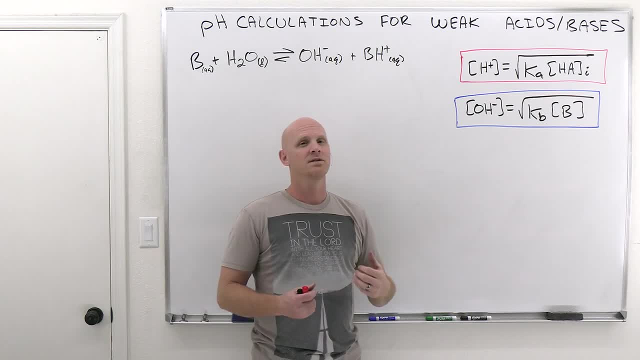 from 14 to get the pH. So, just like we saw with strong bases, so you could calculate the OH pretty readily and take the negative log of the pOH, but you had one extra step compared to strong acids where you had to then subtract from 14.. Same thing with weak bases: We'll have one extra step. 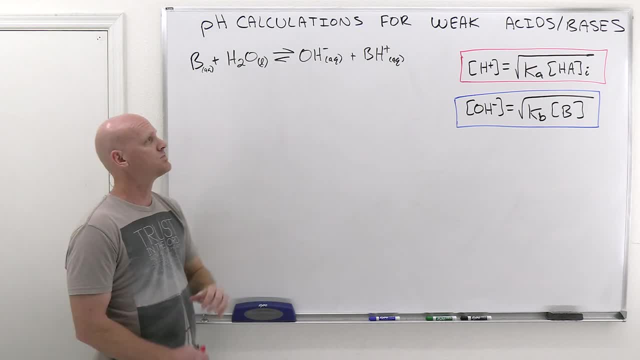 compared to weak acids. Now how do we get there? Well, for a weak base, dissociating water, you have to include water in the reaction. So Bronsted-Lowry's definition of water is that a weak base was a proton acceptor, an H plus acceptor, And that's what the water's job is in. 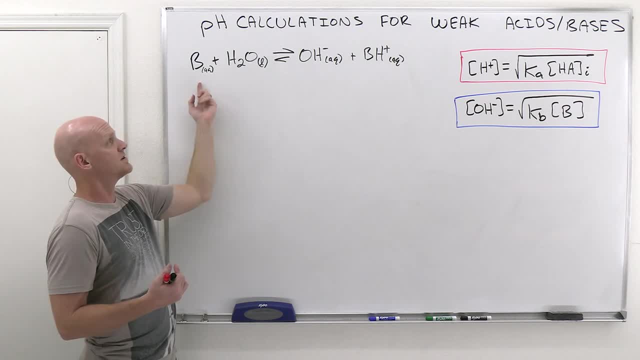 the equation. It's where we're going to get the H plus from. If you don't include it, well then where is the base going to get the H plus from? Well, I don't know. So it has to be part. 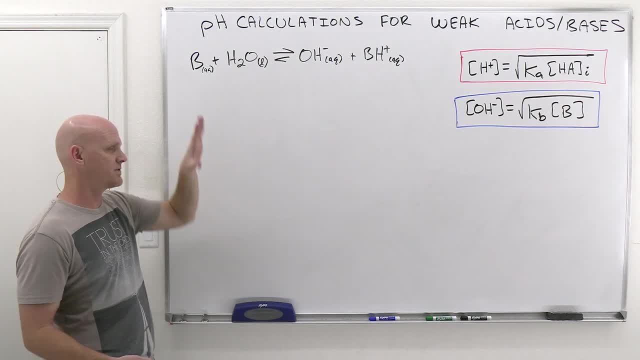 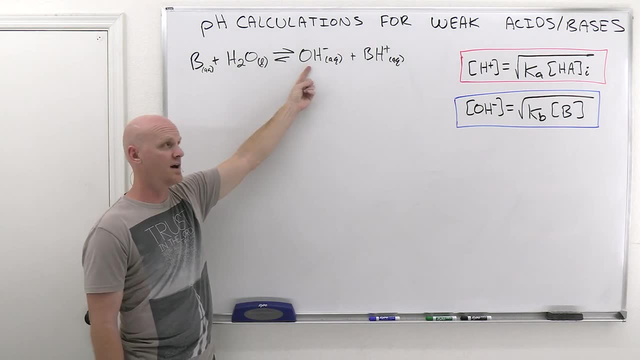 of the reaction. for a weak base, For a weak acid, we have the option to include it or not. But for a weak base you got to include it, And so your base plus water: when you steal an H plus from water you're going to be left with hydroxide And then the base gaining the H plus is going to. 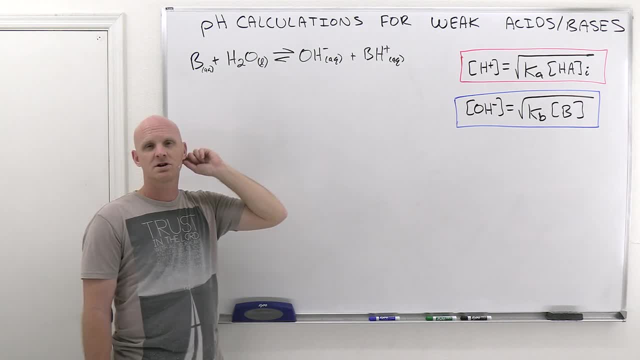 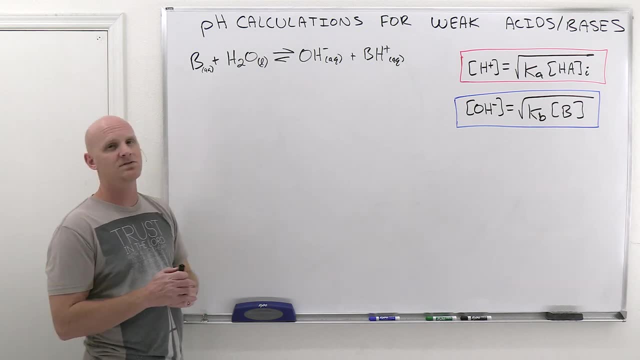 now have an H and a plus charge, So here's generic. So, but what you're going to get is an OH plus. So So, but what you're gonna find more commonly, instead of using B for base, The base will actually use is the conjugate base of the weak acid. 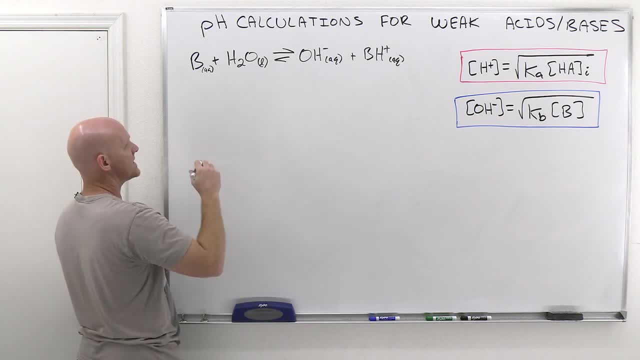 We just showed a little bit ago, And so the acid we showed was HA and the conjugate base was A minus. And so in this case, if you have A minus reacting with water, You're still gonna get your hydroxide as he steals a proton from water here. 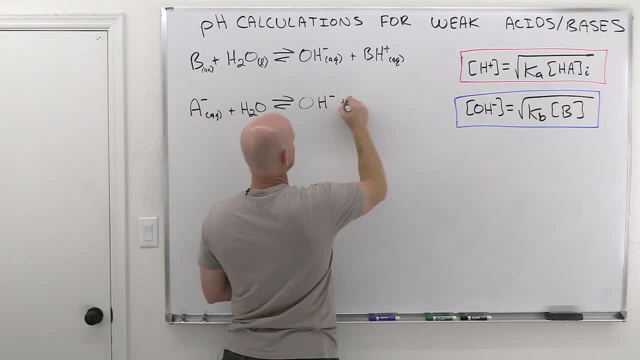 you got your hydroxide left, and as he steals a proton from water, he turns into HA, He has one more H, and when you start out negative and end up with one more positive charge, you end up neutral instead, And so you might also see this written. so now, as 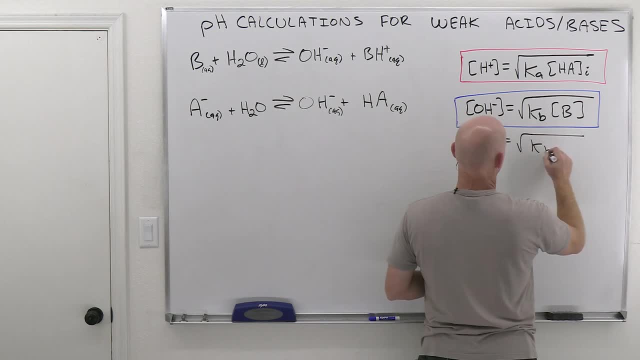 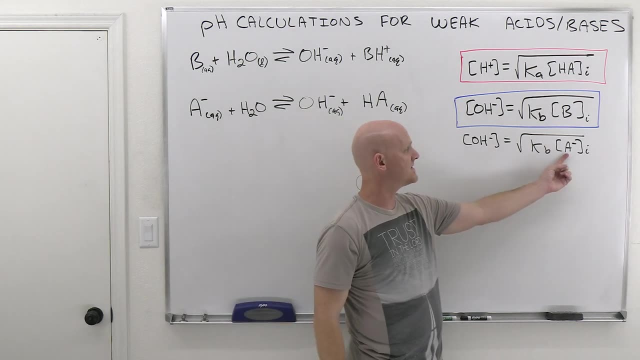 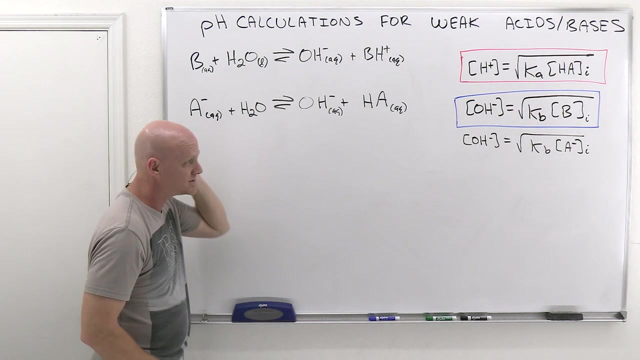 OH minus equals square root of KB Times A minus. You could see it read this way as well. I want to avoid this, though, because a lot, of, a lot of students see that A and they think acid. But this is Really the formula for the conjugate base in this system of abbreviation, so be careful. 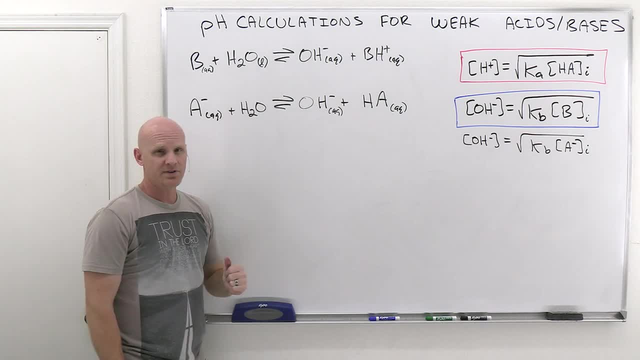 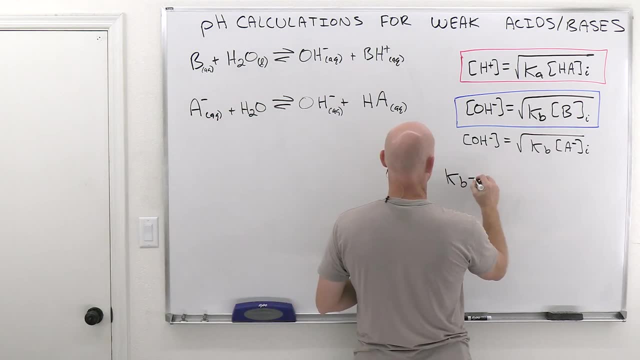 All right. So this is our reaction for a weak base dissociating water. the equilibrium constant of this reaction is called KB. I'll set that up. We'll have hydroxide Times conjugate acid All over Our base concentration, in this case conjugate base, and again. 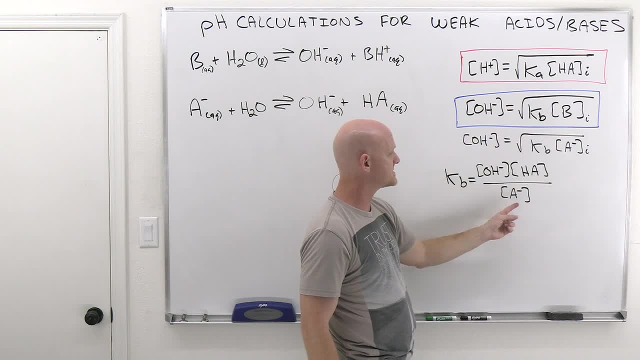 you could have set it up for this one as well, So you might see this written as hydroxide times BH plus all over the concentration of B, same diff. So but it's instructive to write it this way as well, because a second ago we had the KA expression equal to H plus times A minus. 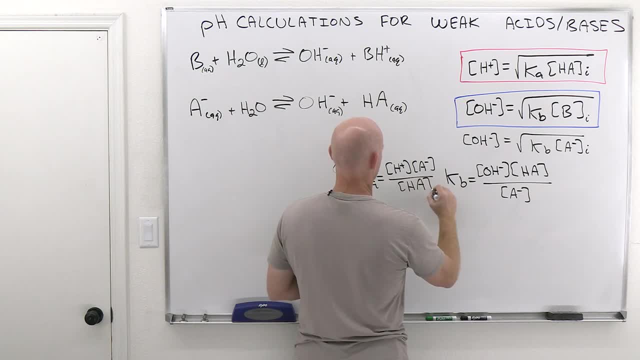 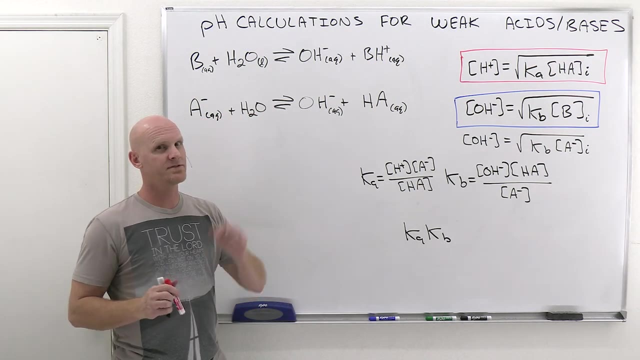 over HA And we'll use this to derive a common expression. It turns out, if you take KA of an acid times KB, specifically of its conjugate base, not just any KB, but the KA of an acid times the KB of its conjugate base, it's always going to multiply out to something. 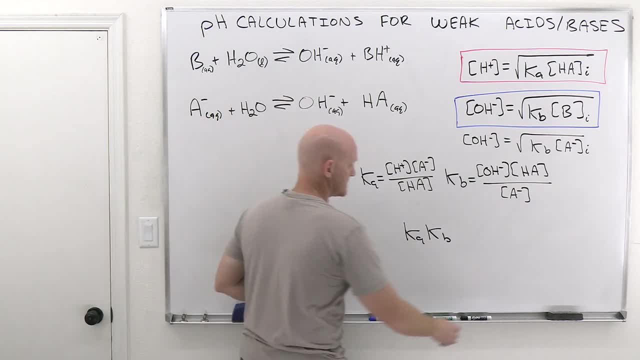 special here. So if you take a look, then we're going to erase this here. We'll take off the KA and the KB here and just multiply these two expressions together, And what are you going to get? Well, you're going to find out that the A minuses here are going to cancel and the HAs 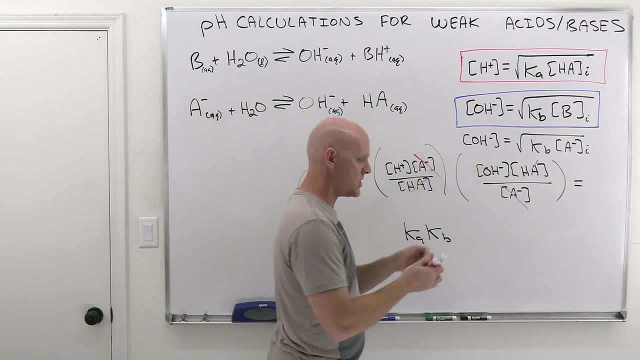 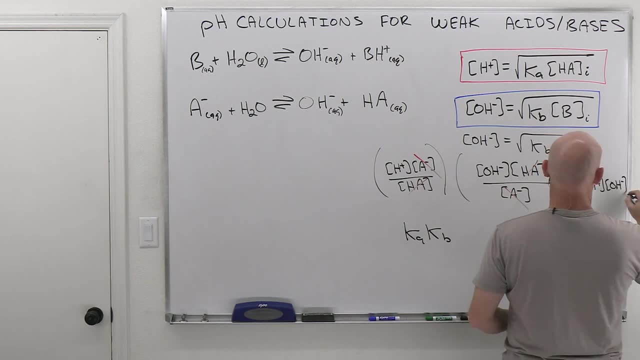 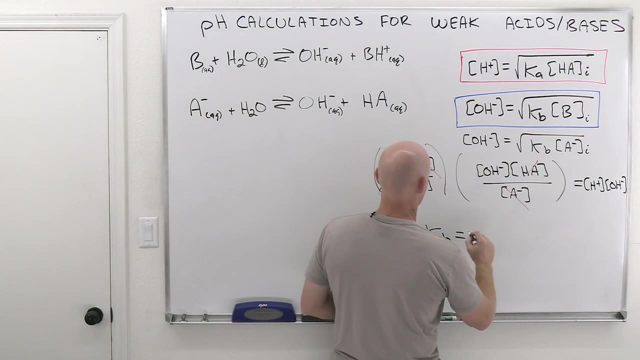 are going to cancel, So you're going to get a common expression here. So you're going to be left with H plus times OH minus. So, if you've already forgotten, H plus times OH minus equals KW 1 times 10 to the negative 14 at 25 degrees Celsius. And so it turns out for any conjugate. 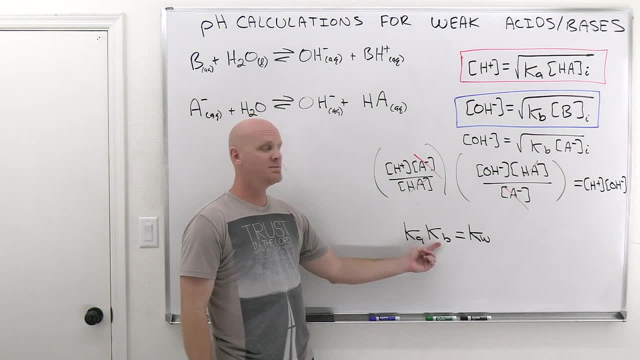 acid base pair. the KA value of the conjugate acid times, the KB of the conjugate base always multiplies out to give KW. So this is important. So we looked at KA values a little bit ago and we said that oh the higher. 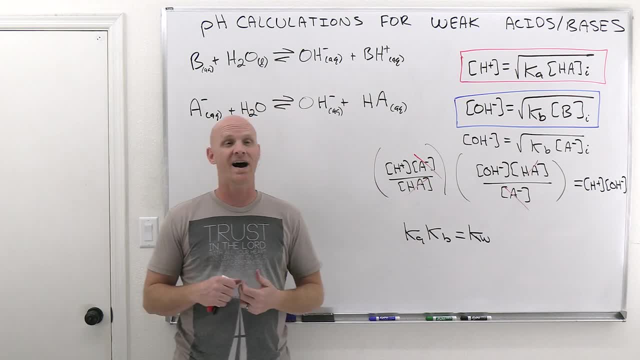 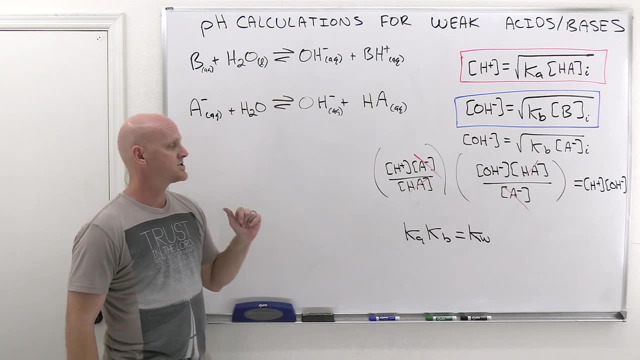 the KA, the stronger the acid. Well, we can look at KB values for bases too, And the higher the KB, the more products you get and the stronger the base. So higher KAs mean stronger acids, higher KBs mean stronger bases. So, however, there's a relationship between a weak acid, 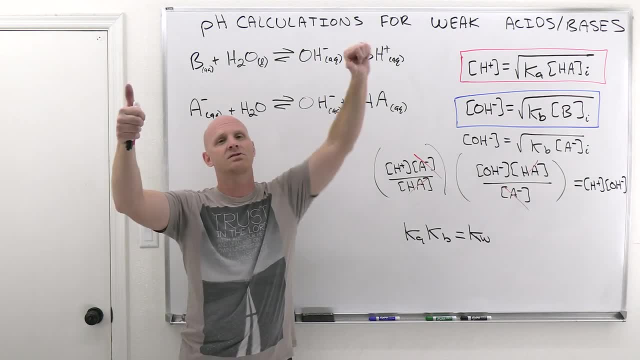 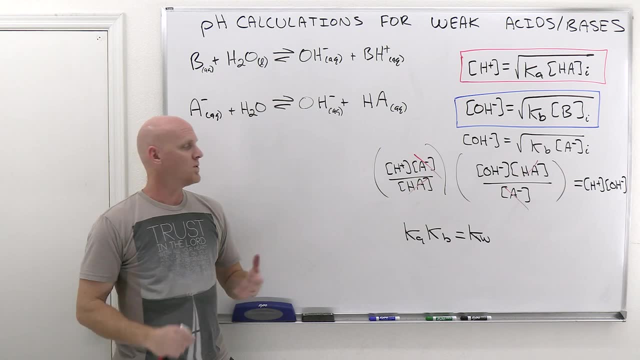 and its conjugate base. And the stronger an acid, the weaker its conjugate base, and vice versa. We saw this when we talked about the binary acid trend and the oxoacid trend and things of this sort. Well, here you can see it mathematically, because if you have a stronger acid, it's going to have. 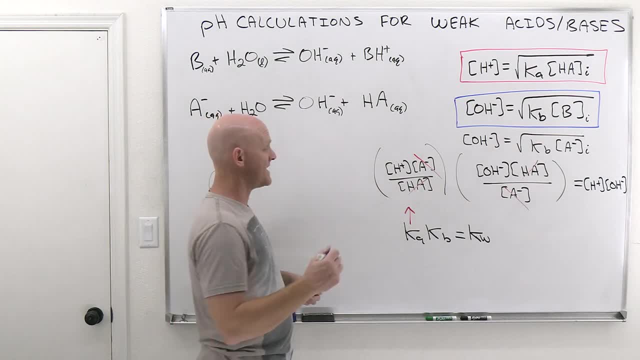 a larger KA value. And if it has a larger KA value, well then the conjugate base is going to have to have a smaller KB value, so that when you multiply them together you still get 1 times 10 to the negative 14.. And so now, mathematically we can see that the stronger an acid, the weaker 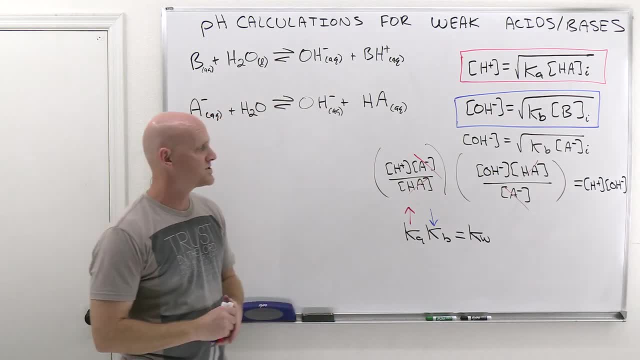 its conjugate base and vice versa. So I just wanted you to see it both mathematically as well as just the reasoning. All right, So if I give you a bunch of numbers, I'm going to give you a bunch of numbers. 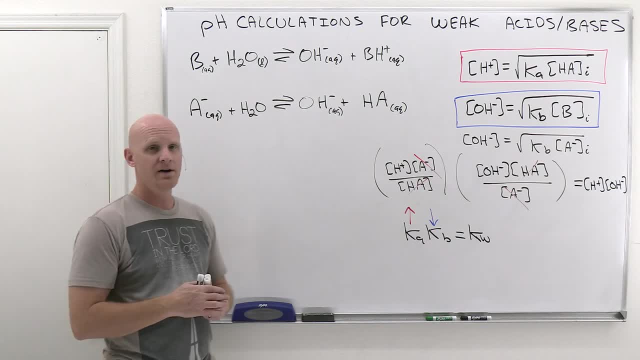 I'm going to give you a bunch of KA values now And, if you notice, we had KA values for HF, for acetic acid and HCN And we said that HF was the strongest of those three acids because it had the highest KA. 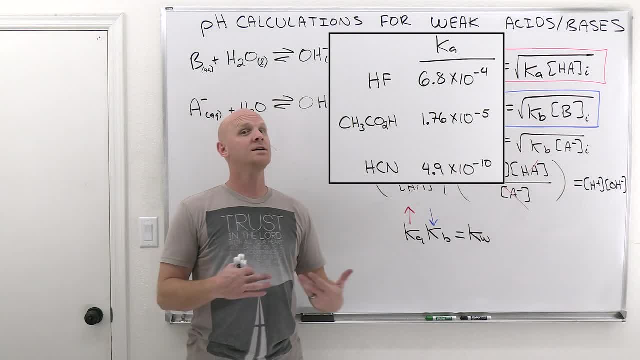 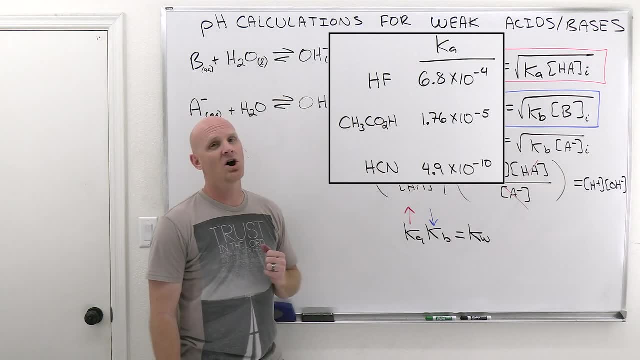 value. Well, you could automatically infer that F- would be the weakest of the conjugate bases, because it had the strongest conjugate acid. Because the strongest conjugate acid will have the weakest conjugate base. So now, not only will KAs give you a way of comparing acids, 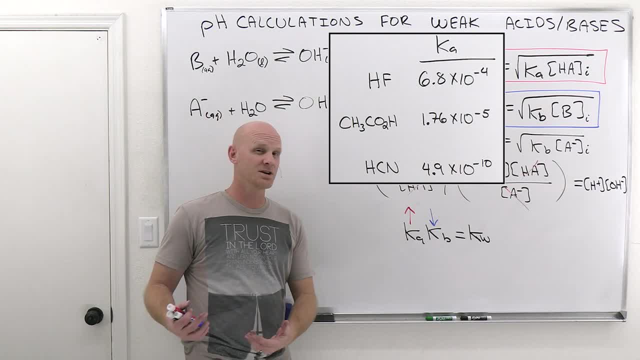 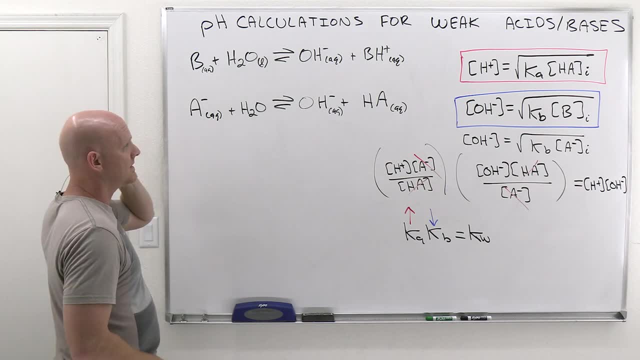 they'll also give you a way of having the opposite relationship for comparing the conjugate bases. All right. Same thing if I give you KBs and you want to compare the conjugate acids instead, All right. So the question we're looking at here is: what is the pH of 0.1 molar solution of? 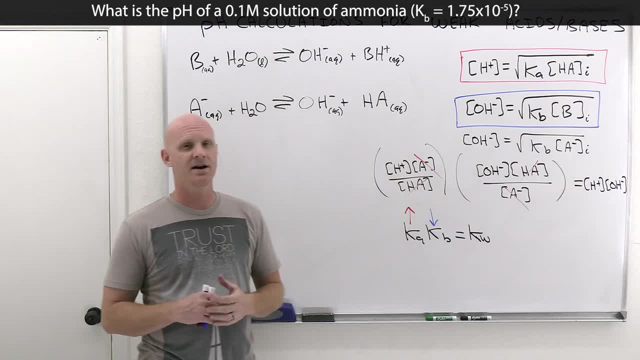 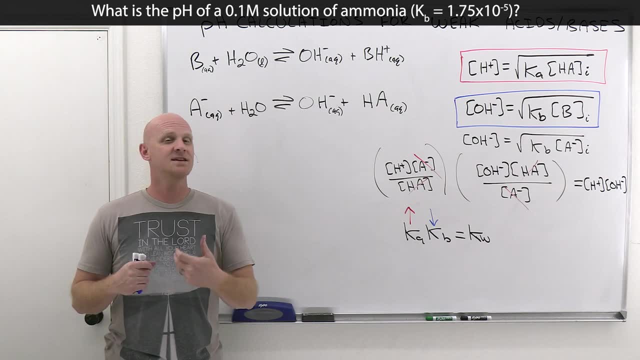 ammonia And the KB is given as 1.75 times 10 to the minus 5.. I chose this example on purpose. It's still 0.1 molar weak base, But instead of acetic acid, which had a KA of 1.76 times 10 to the minus 5,. 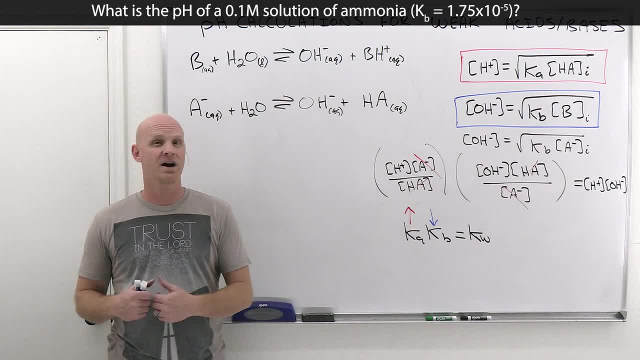 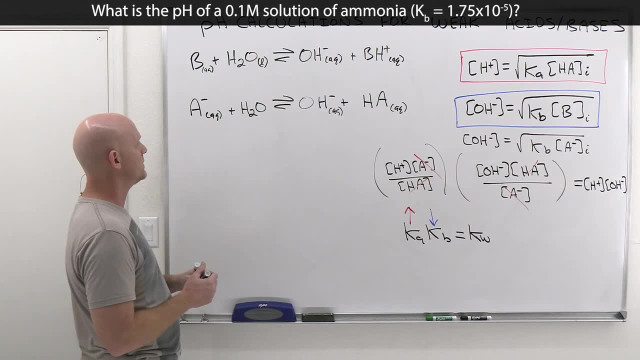 ammonia has a KB of 1.75 times 10 to the minus 5.. Almost exactly the same numerical value And the reason I chose that is because it essentially is going to end up looking very similar, when we solve it, to the one we did earlier for the weak acid And if we set up the ICE table. 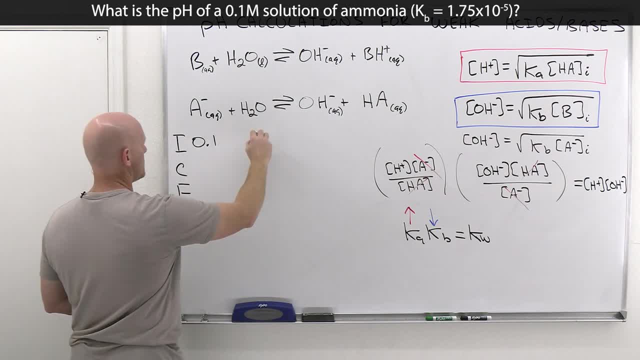 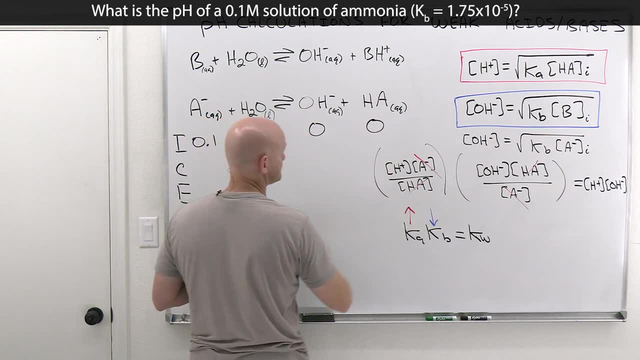 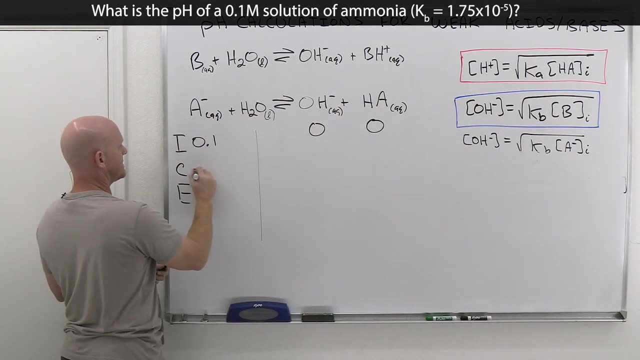 here we initially start with 0.1 molar A minus. We'll ignore the water, since he's a liquid and doesn't show up in the KB expression anyways, And then we'll have a zero here and a zero here, And then the amount that associates is going to be X. So minus X on the reactant side, plus X. 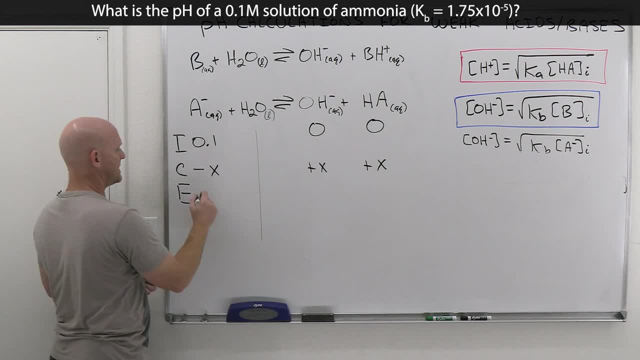 on the product side, 0.1 plus a negative X is 0.1 minus X. This should be looking really familiar. Zero plus X is X, Zero plus X is X. But in the case of a base, bases don't produce. 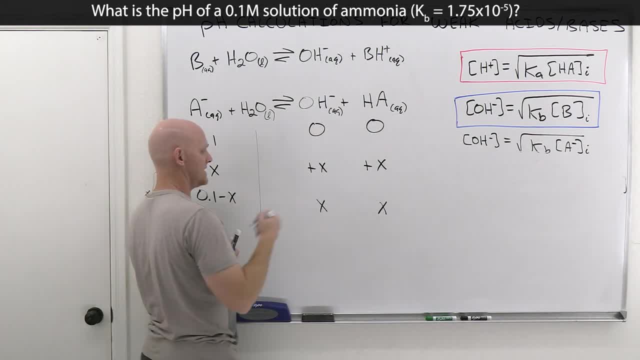 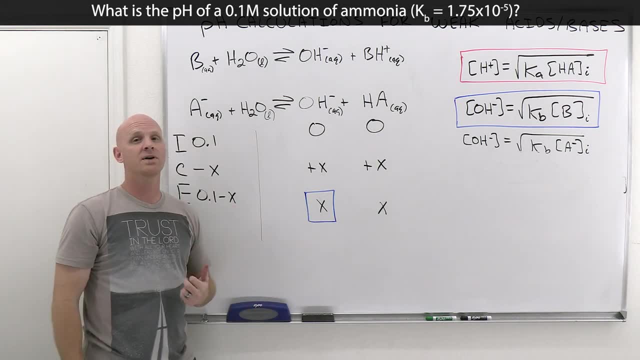 hydronium or H plus They produce hydroxide, And the whole point in setting this up is for what goes in this box right here. And so what goes in this box turns out as X, And when we solve for X, 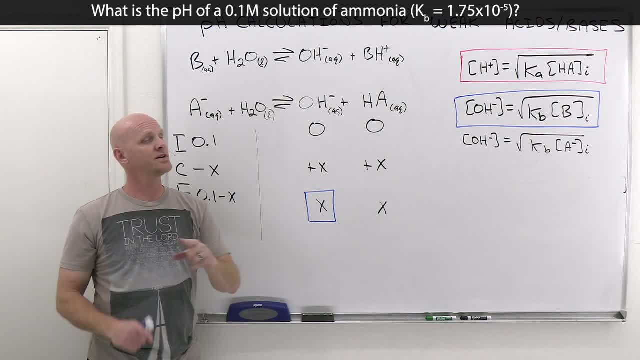 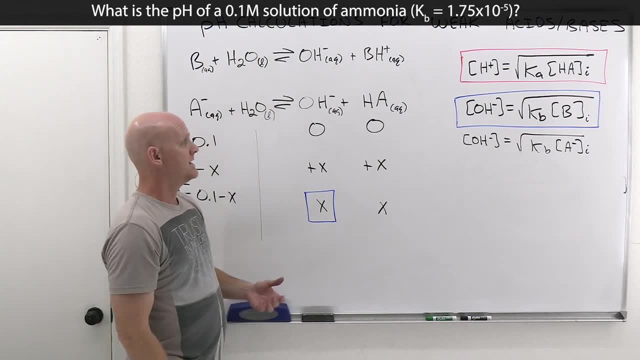 that is the hydroxide concentration, And we'll take the negative log not to get the pH directly, but the pOH, And then we'll subtract from 14 to get the pH All right. And again, if we set this up, then your 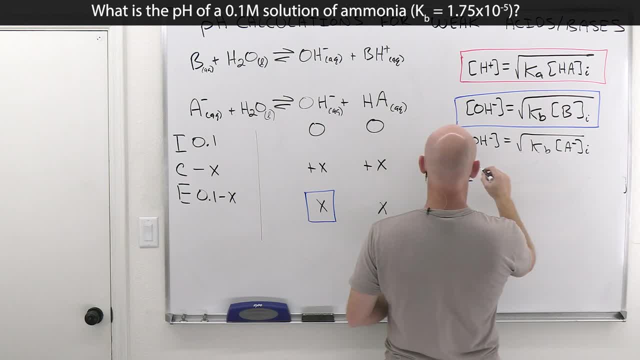 KB is equal to OH minus times HA, all over A minus, And in this case we're given that the KB value is 1.75 times 10 to the negative 5.. That's going to equal X times X, So X squared. 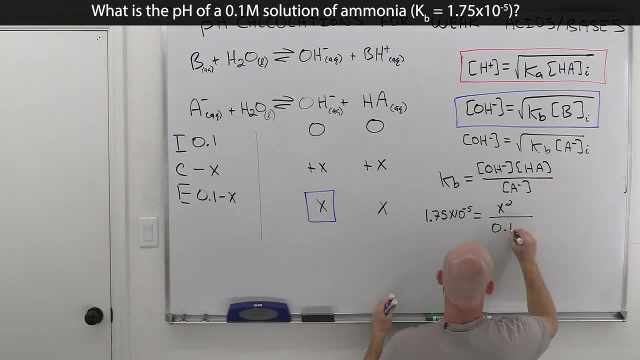 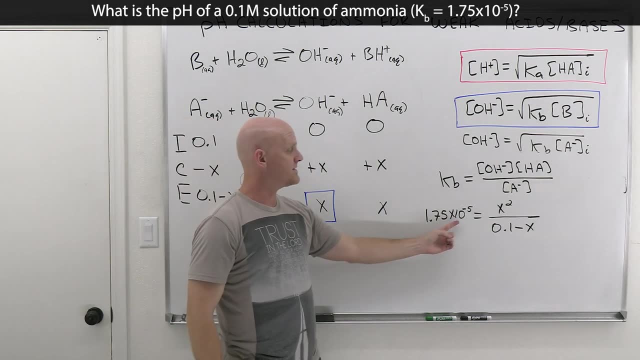 All over 0.1 minus X. And notice this is essentially the same equation we had for acetic acid a little bit ago: Instead of 1.75 times 10 to the minus 5, it had 1.76 times 10 to the minus 5.. 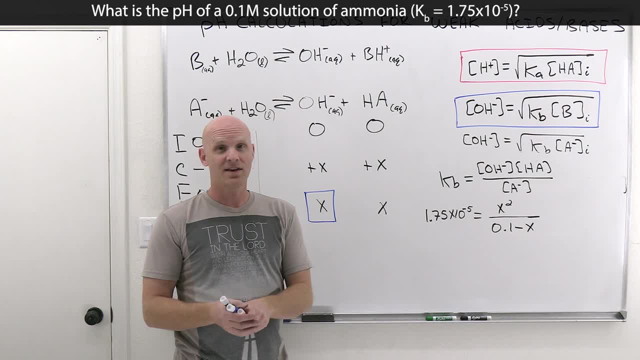 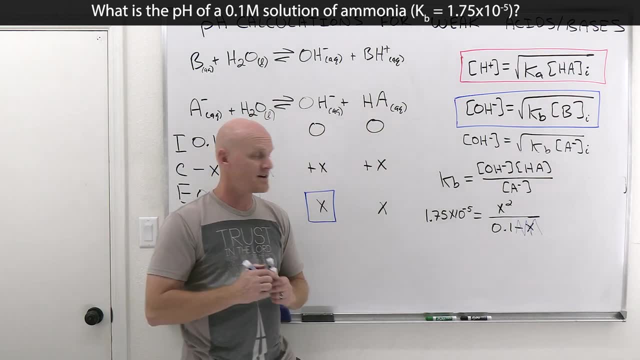 But the rest of the equation was identical And, as a result, we're going to get the exact same solution for X. We're going to do the same thing we did before. We're going to ignore the minus X here, knowing that most weak bases are going to dissociate less than 5%, So X will be less than. 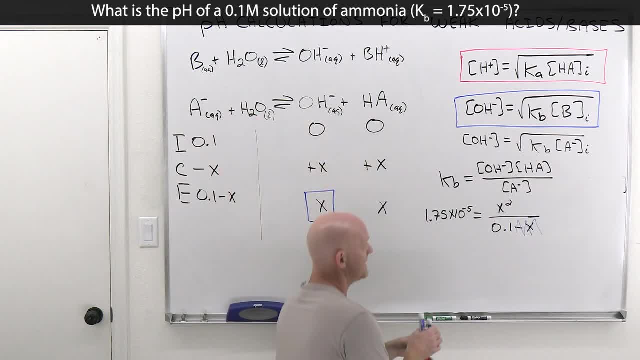 5% of 0.1.. We know it will. We already solved this one before And we're going to do the same thing And in fact we're going to get the same value for x here. We'll multiply this up by 0.1.. So we'll have. 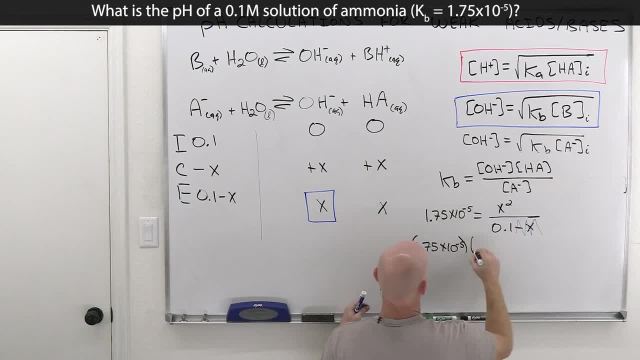 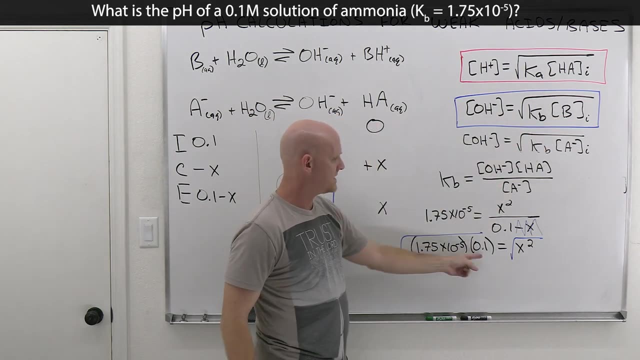 1.75 times 10 to the negative, 5 times 0.1 Equals x squared. We'll take the square root of both sides. Notice, that's where our equation comes from. we have the Kb now times the base concentration Multiplied together. take the square root. it gives us x, which is not h plus. it's now, Oh, h minus. 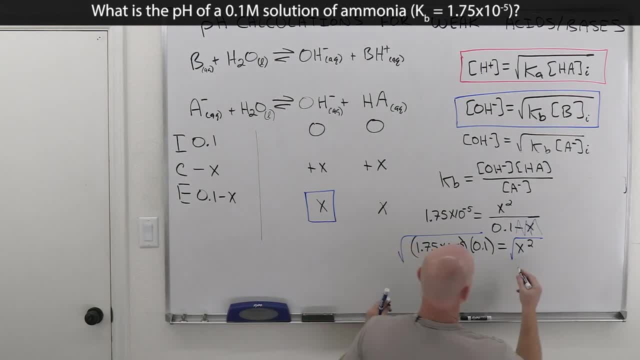 But it's still going to equal 0.0013 again. But now that doesn't equal h plus, that equals, Oh, h minus. and so when we take the negative log and get 2.9.. We don't get the pH, we get the p, Oh. 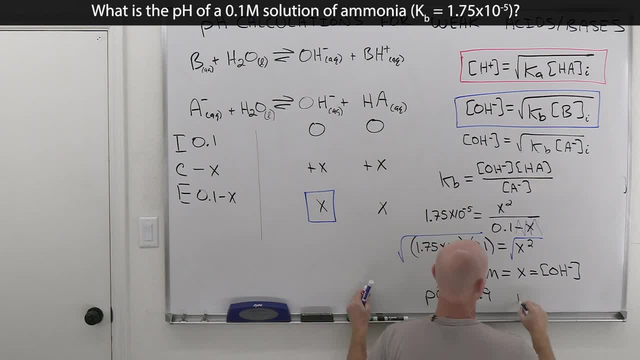 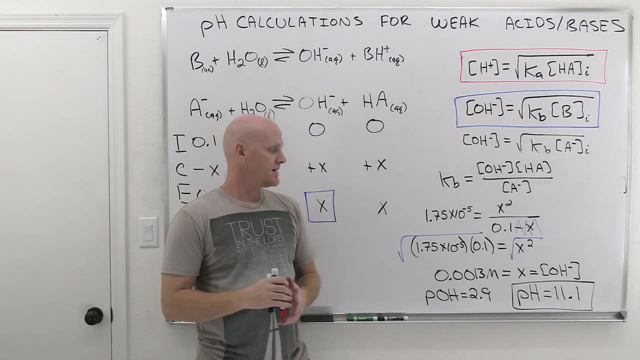 H is Equal to 2.9.. And so if we want to solve for the pH, we got to subtract from 14, and 14 minus 2.9 Is 11.1. so one extra step At the end to get the pH of a weak base. 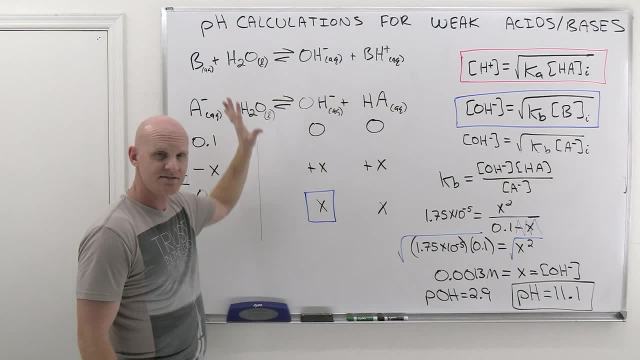 Cool. we did the whole ice chart. We set it up again. This is instructive. I think it's useful for you to know how to do this, But at the end of the day, you want to get to the point where, for most weak bases, 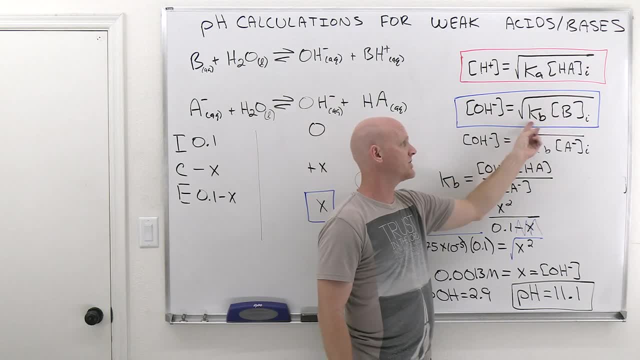 Probably just going shortcut. you're like: well, they gave me the Kb, They gave me the base concentration. I'll just multiply them together and take the square root and that's my hydroxide concentration. I'll take the negative log- you got a negative log of that- and get the pOH. 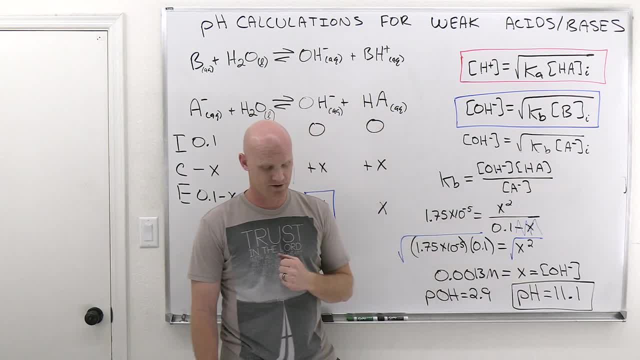 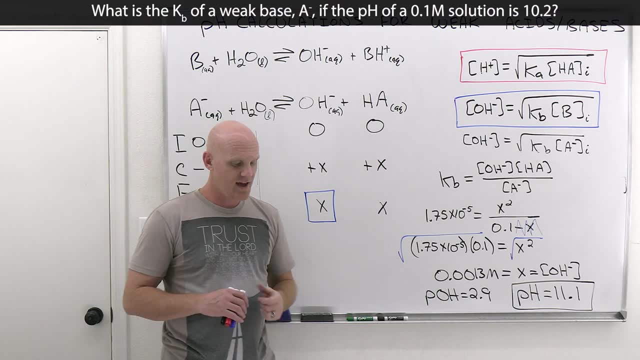 And then I'll subtract that from 14 to get the pH. All right, we've got one more question here for weak bases, Excuse me, and that is: what is the Kb of a weak base, a minus, if the pH of a 0.1 molar solution is 10.2? 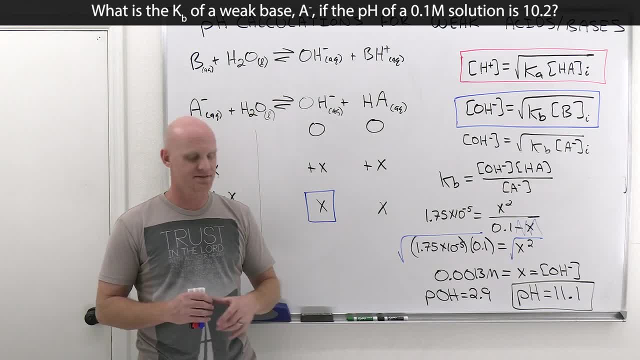 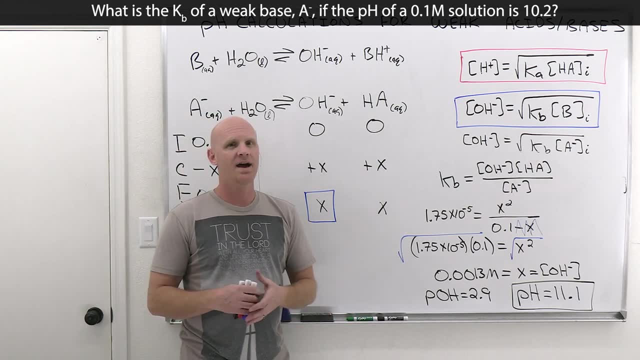 This is probably the hardest question we're encountering in this section, So but it really is not much more challenging than the one- the analogous question- we did for finding the Ka of a weak acid, But in this case you're given that the pH is 10.2. 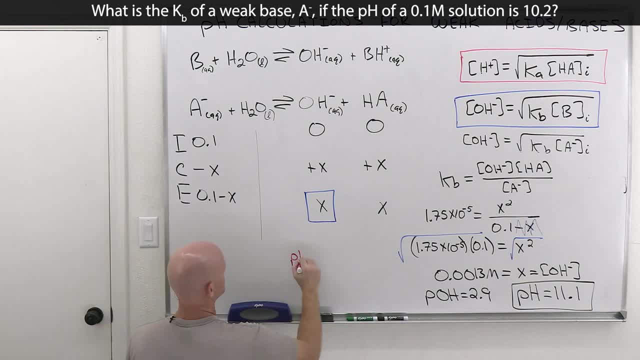 Let's let's reason this out for a second. So the pH Is 10.2. well, that means What I really want out of this is: I want what goes in this box, I want X, and X is the hydroxide concentration. How do I get there from a pH? 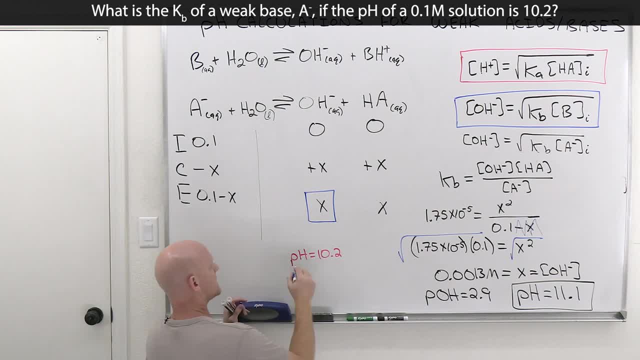 Well, I can get there in a couple different ways, But probably the most readily, readily, readily available way to get there, or the easiest way to get there, is to subtract 14 and get the pH- I'm sorry, the pOH- of 3.8, and then they get the. 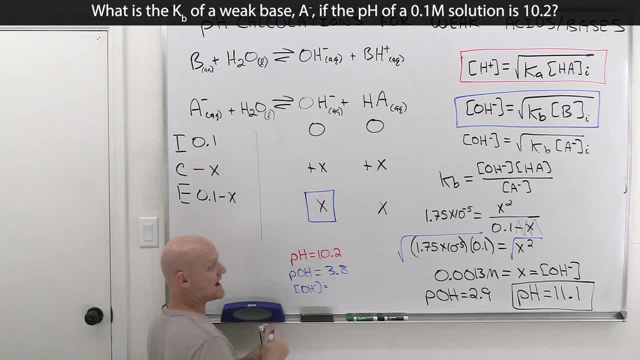 Hydroxide concentration, which is going to be 10 to the negative 3.8. so- and you know what- that's not proper. but you know what I don't care. It's not what I'm actually looking for. It's not going to be one of my multiple choice answers if I'm taking a 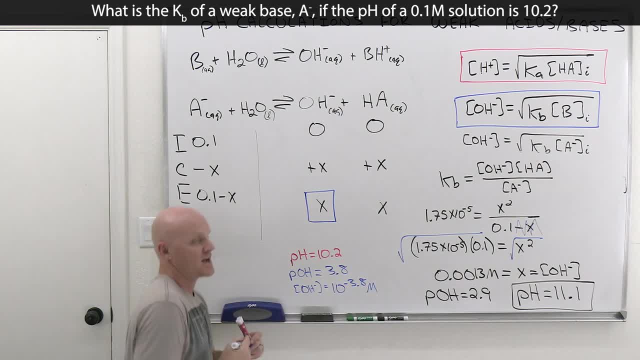 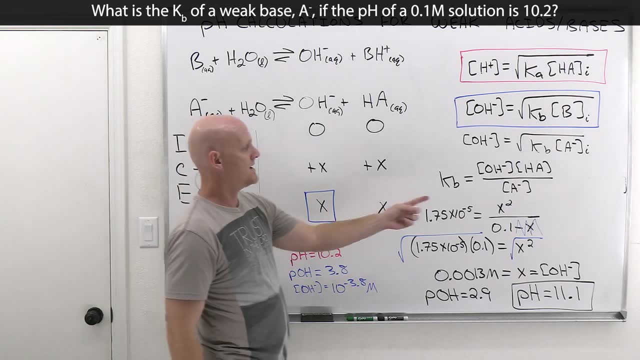 multiple choice test, but 10 to the negative 3.8 molar. I Can plug that into my calculator and have it tell me what looks like, but I'm just actually going to plug that into my equation here, so We can see that our Kb is just going to be x squared over 0.1 minus x, where X just happens to be 10 to the negative. 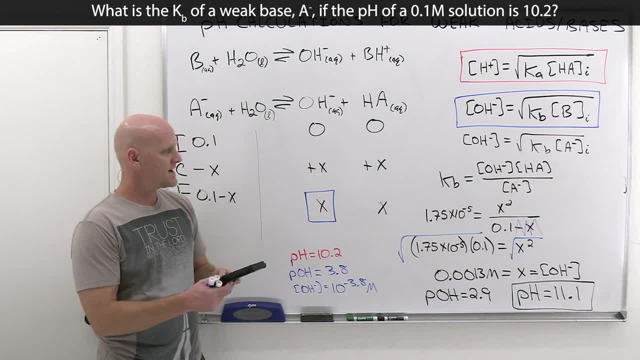 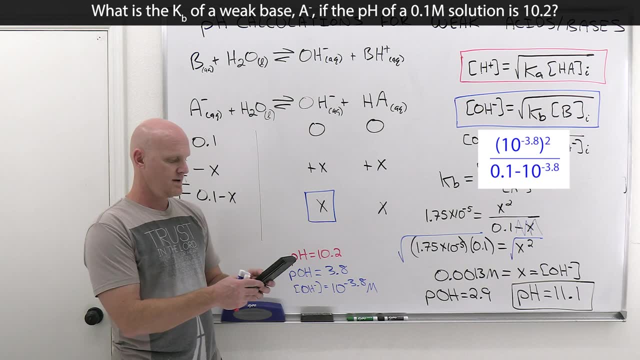 3.8, and so in this case case I'm going to take 10 to the negative 3.8 squared, So 10 carat negative 3.8 squared divided by 0.1, minus that value, which probably will be insignificant again, but again I'm not solving. 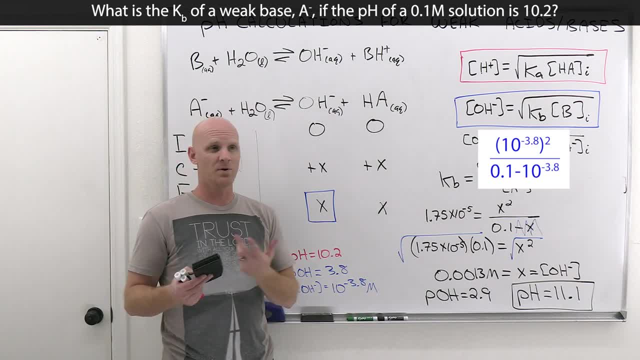 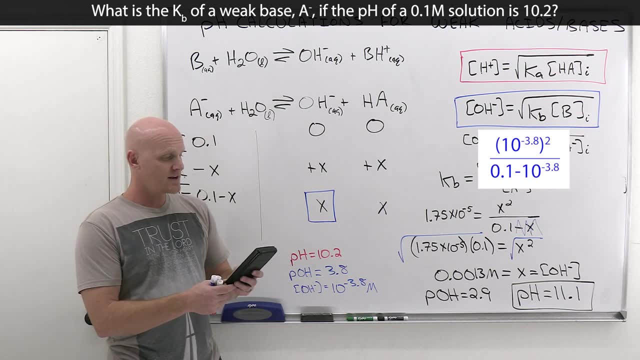 for x. So by substituting it in, it doesn't actually, you know, mean I don't, I'm not going to have to solve a quadratic or anything like that, So I might as well include it, just to get a more exact answer. So 10 to the negative, 3.8 squared, divided by parentheses, 0.1 minus 10 carat negative. 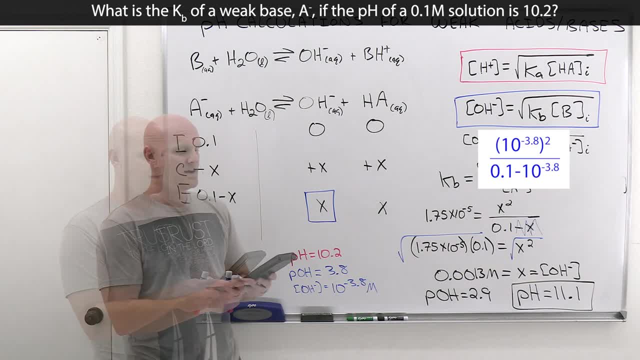 3.8- end parentheses- gets me 3.6 times 10 to the negative 14.. It just seems so small that I didn't think it was the right answer. So, but in this case we're going to get a KB value of 3.6 times. 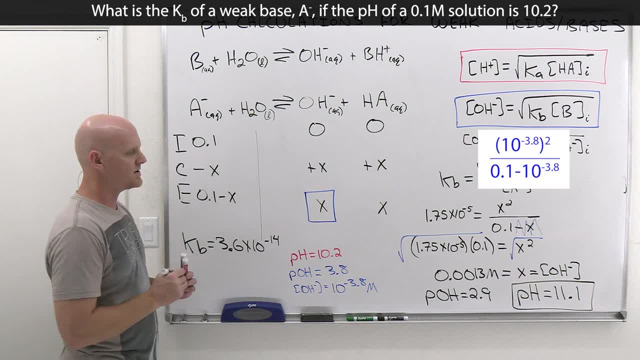 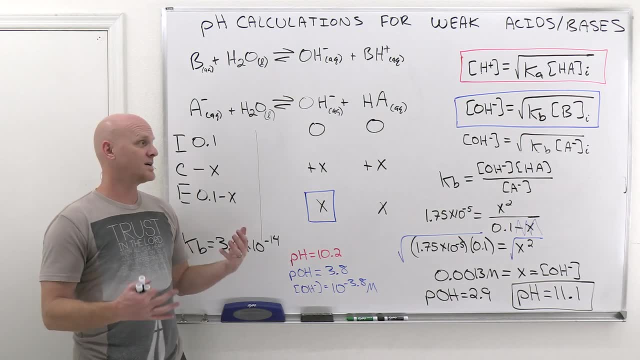 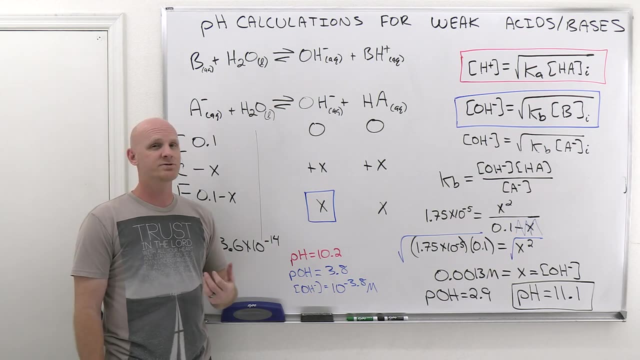 10 to the negative 14.. We have a fairly weak base on our hands in this case. Cool, And this is how it works Essentially. you know, one extra step for weak base- that's compared to weak, And this last one again for whatever reason. that one extra step is super tricky. It's an. 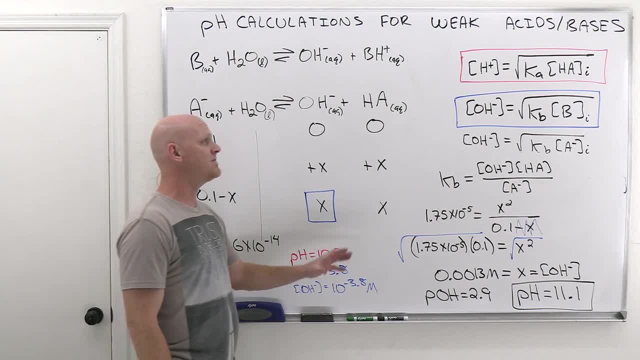 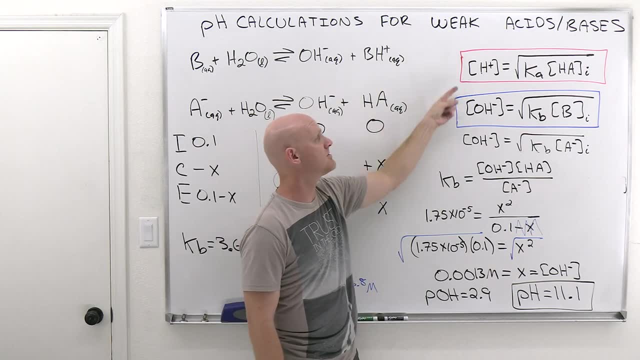 extra step at the beginning and the end. So, but this is what it takes. But at the end of the day, I want you to get to the point where, for any weak acid or weak base, you're asked to find the pH, that you immediately think about one of these two equations. And so now again, it really is an ice. 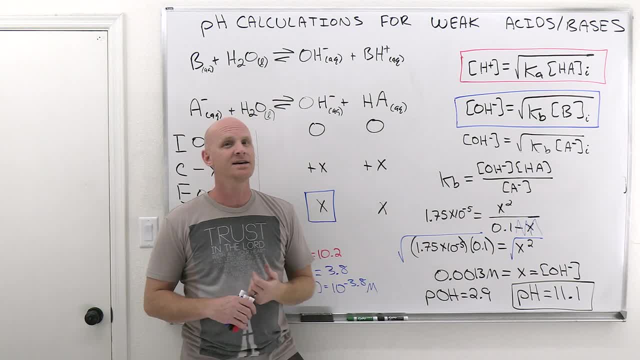 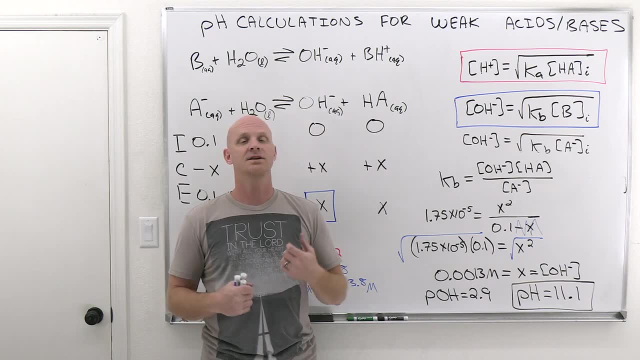 table and all this. you know this process that we've learned how to do for equilibrium calculations. However, we now have quick ways of calculating the pH for a strong acid dissociates completely And a strong base dissociates completely, But now also for a weak acid or weak base. 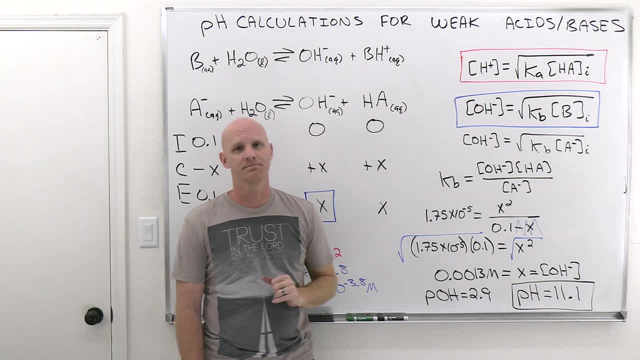 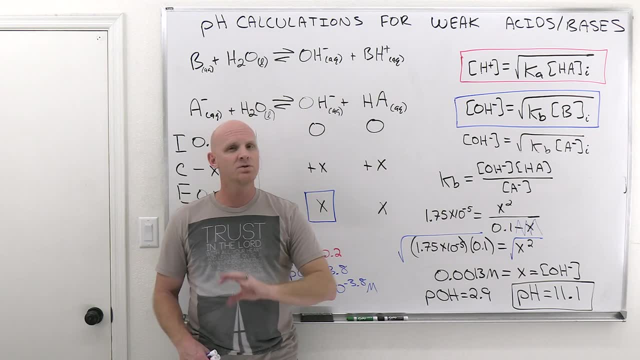 we have a very quick formula that's going to work more than 90% of the time And it's going to be important. You have to get really good at pH calculations And one of the big things is that you're going to have numerous types of solutions by the time. all of a sudden, 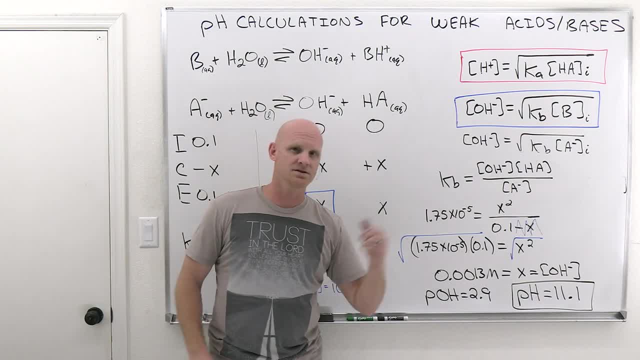 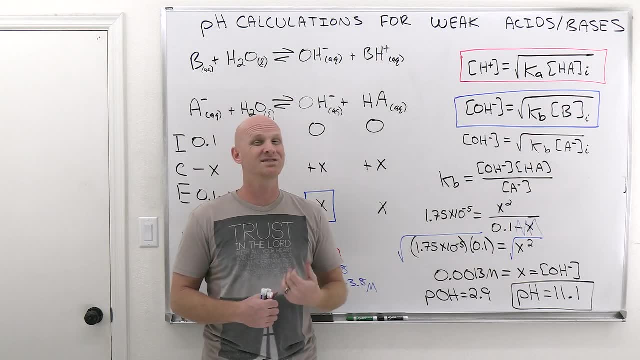 done for calculating the pH. You might have it for a strong acid or a strong base, for a weak acid or a weak base, or you might have it for a buffer, or you might be doing a titration, And so half of the problem is going to be even realizing. 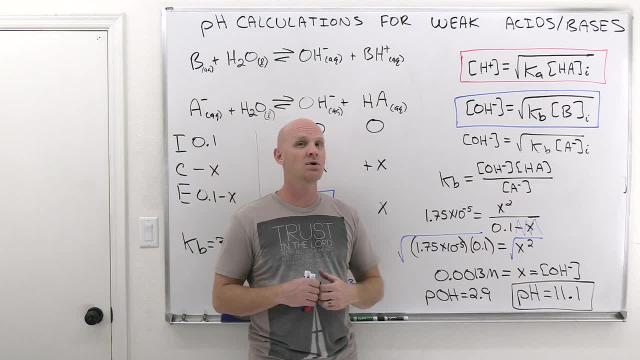 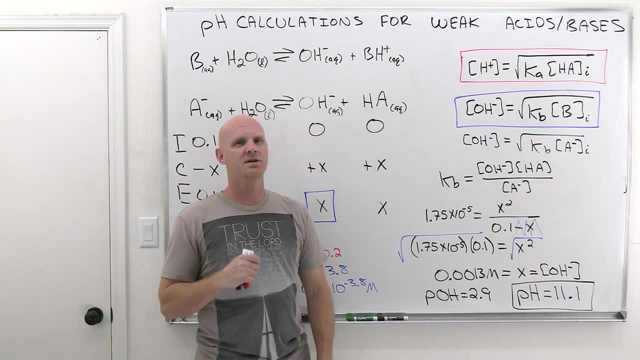 what kind of solution you have and then what's the proper format for actually calculating and determining pH. So strong acid dissociates completely, you'll get the H plus concentration very directly and then take the negative log and get the pH Strong base. you'll be getting the OH. 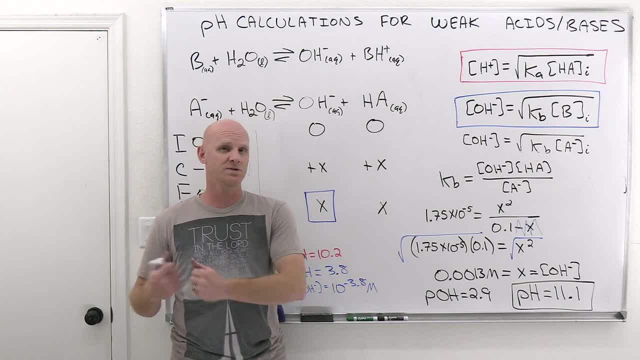 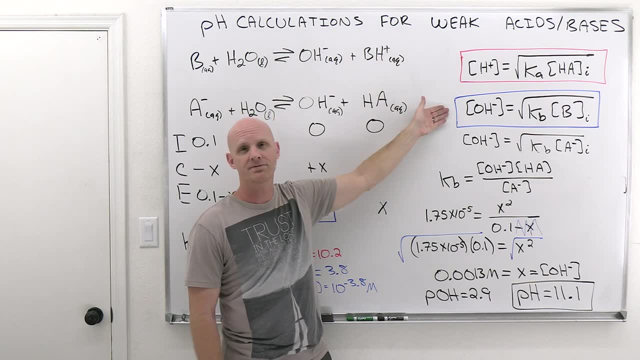 minus concentration very directly and taking the negative log and get the pOH subtract from 14.. Weak acid: we got a formula for the H plus And once you solve for that, take the negative log and get the pH. Weak base, we have a formula for the hydroxide. Once you. 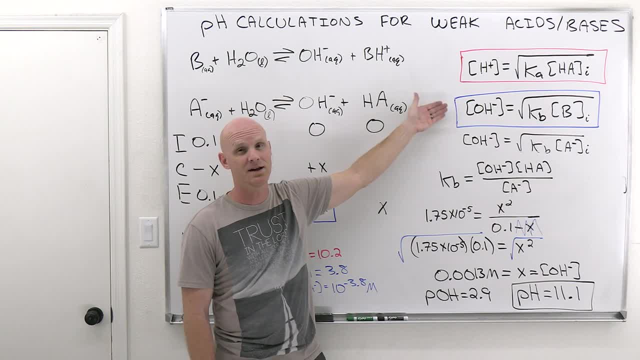 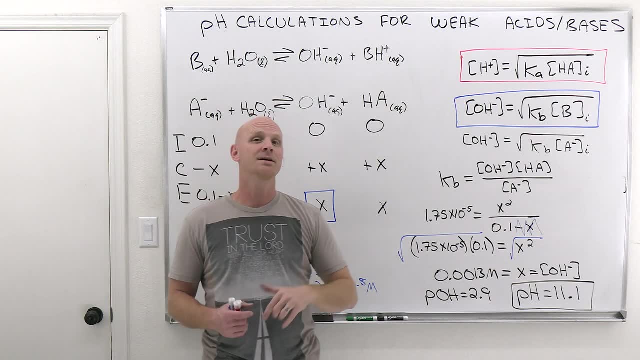 solve it. you'll get the negative log. you get the pOH and subtract from 14. To get the pH, And that's four out of the five standard type solution. We'll deal with buffers in a little bit and then we'll see that titrations turn into most of these. But again, buffers and 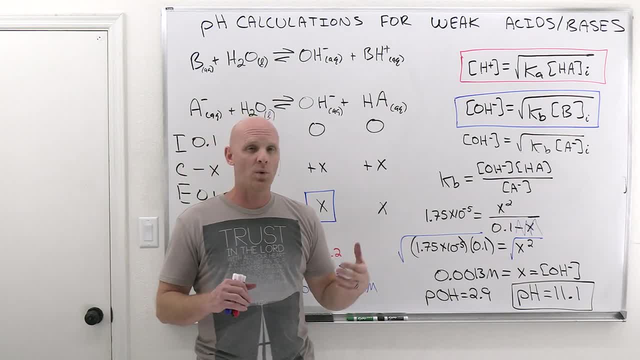 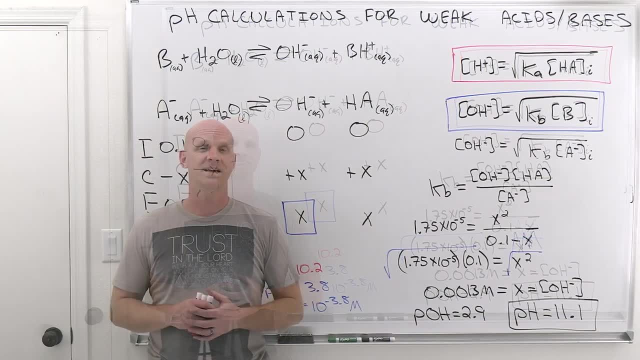 titrations in the next chapter. All right, we've got one more topic to talk about in the next lesson. That's going to be talking about the acidity and basicity of salt. Now, if you found this lesson helpful, that thumbs up button goes a long way to making. 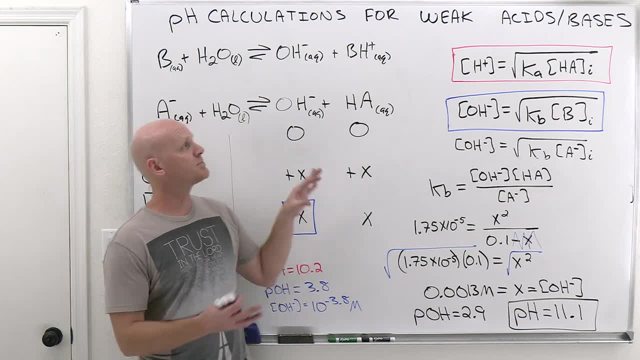 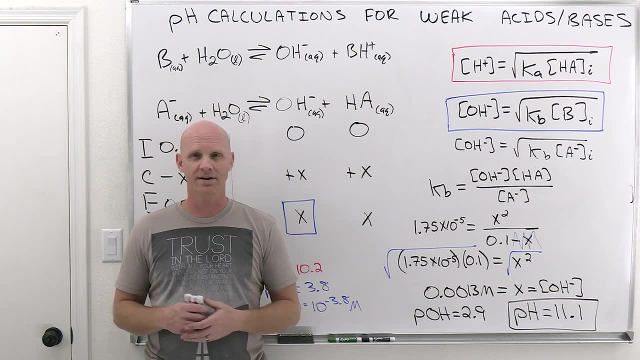 sure other students get to see this lesson as well. And if you're looking for practice problems on weak acids and bases or acids and bases in general or anything in general chemistry, my general chemistry master course includes over 1200 practice questions. final exam: 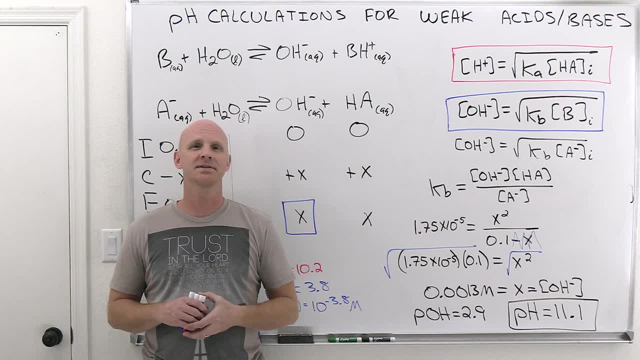 rapid reviews. I'll leave a link in the description. A free trial is available. Happy studying.